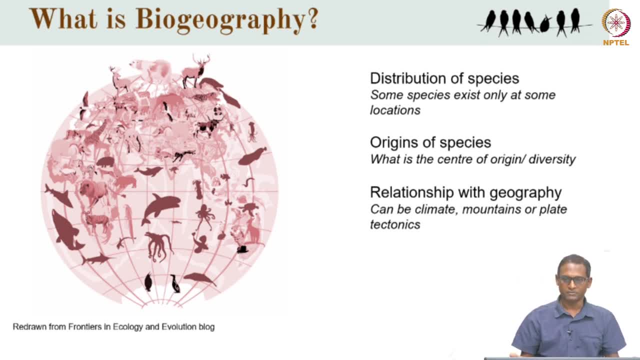 giraffes everywhere, and that is essentially what biogeography is, that some species exist only at some locations. Biogeography is also the study of trying to understand the origins of species. what is the center or of origin or diversity and the relationship with geography? 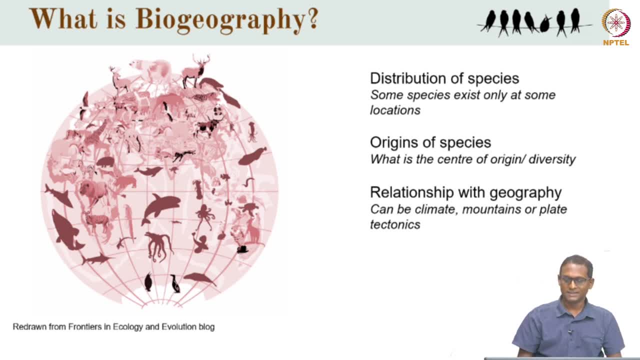 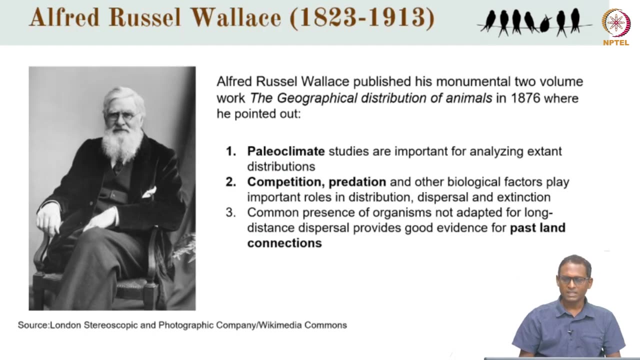 which is, you know, the geography, the biogeography part, And this relationship with geography can come from climate, it can be mountains or plate tectonics, and we will talk about these aspects in detail. So, in some ways, the idea of biogeography and a 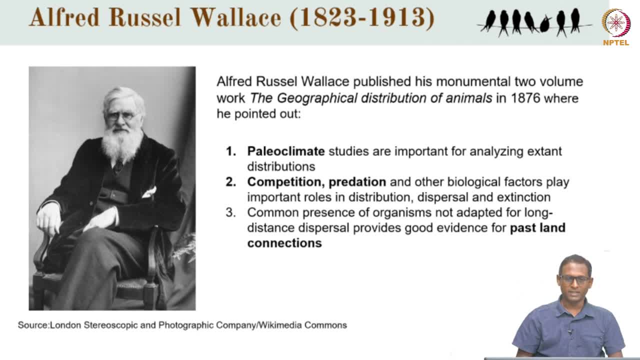 lot of the research on biogeography was heralded by Alfred Russel Wallace and many of you may know Wallace as the co-proponent of the theory of evolution. And, of course, I think people can read up more about Wallace and his monumental contributions. 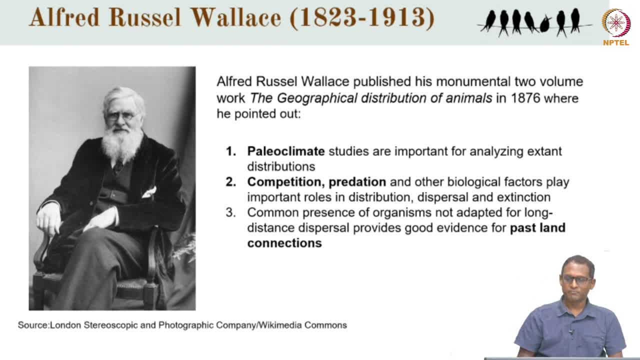 in the book that is there on the slide, But he also. the main contributions were that he pointed out that historic climate, or paleoclimate, is actually important for analyzing or understanding the current distributions of species, and other factors like competition, predation and biological factors play an important role in dispersal and extinction of species as well. 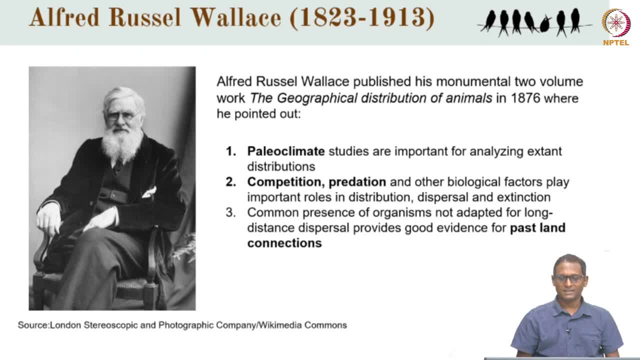 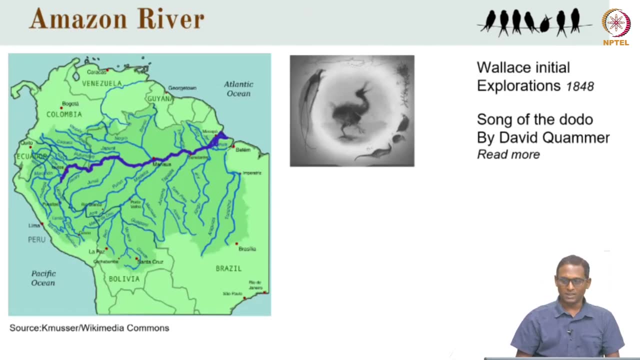 And in some cases, what also happens is that the current distribution of species is because of some historic conditions, like past land connections and so on. So if you want to read more about Wallace, I think the best source of information, which is very easy to read, would be this book. 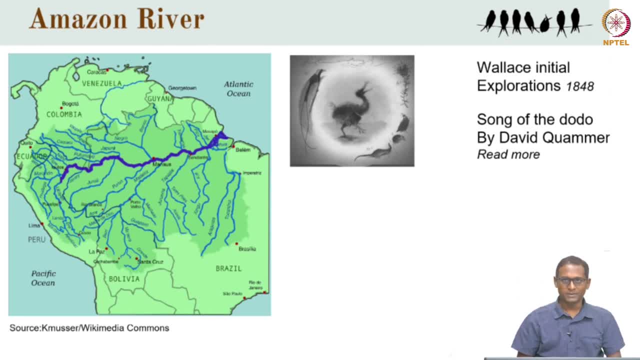 Song of the Dodo by David Quammen. I would recommend anybody interested to know more about him and biogeography to read this book. It is very fascinating, But for the purposes of this talk I will quickly summarize it. So Wallace was actually. he spent a lot of time exploring the 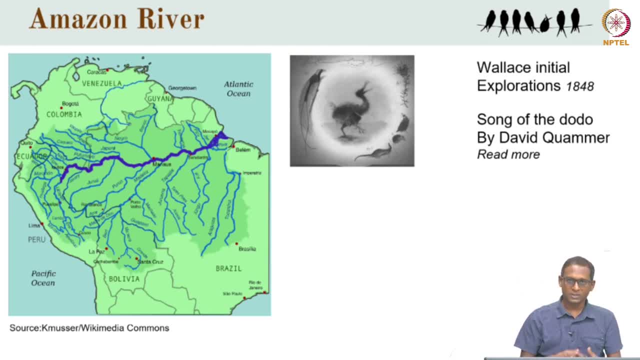 different parts of the world And in 1840s he spent a lot of time exploring the Amazon And he went into parts of Amazon which were not well studied And he spent a lot of time documenting the flora and fauna of these areas and describing several species. And in those days, as is the case, 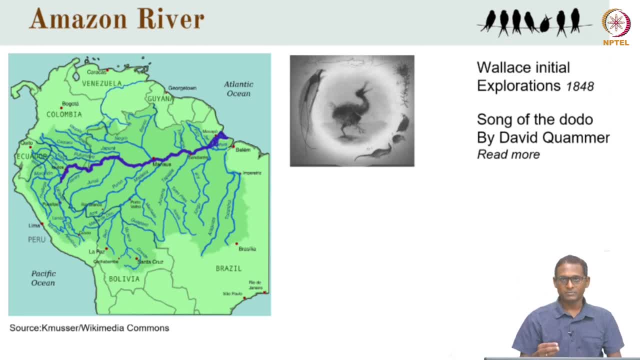 even for some taxa. today, these museum specimens, specimens- have to be deposited somewhere And that is the actual record of the description of a new species. And when Wallace had done a lot of work in Amazon, he was ready to go back to London and 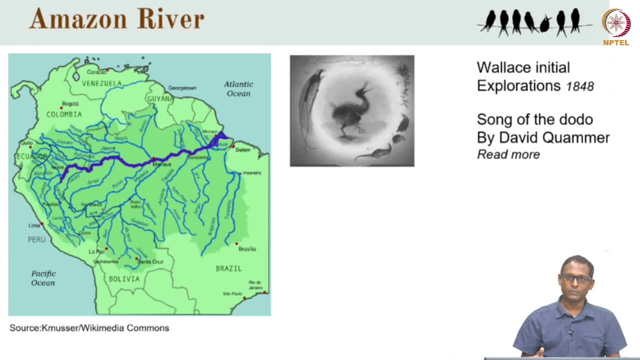 submit his specimens And unfortunately, what happened was during the journey, his ship actually sank with his life's work And that you can imagine was the end of his life's work And that you can imagine was the end of his life's work And that you can imagine was the end of his life's work And that you can imagine. 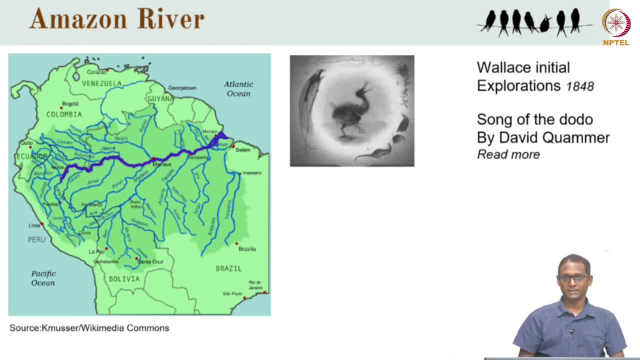 can be quite a tragedy, And it's also a tragedy economically for explorers at that time, because some of them also sell copies of their specimens to other museums And that is how they support their subsequent explorations. So this was quite quite disastrous for Wallace. 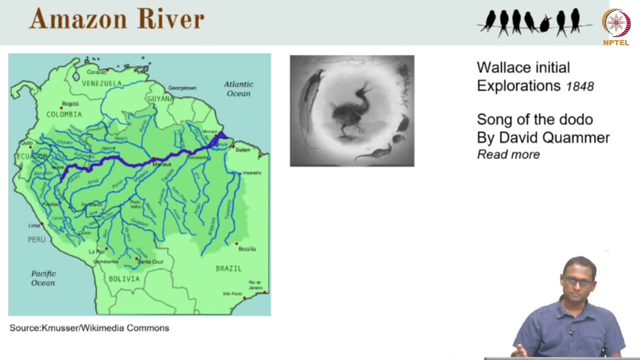 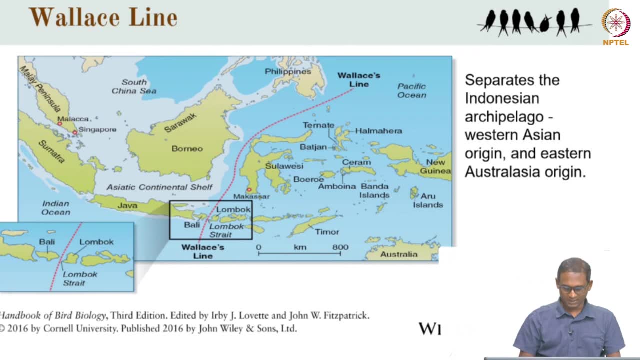 but somehow he picked himself up and then he went on And he went to Southeast Asia next after the Amazon was there. The Amazon was the same place selling specimens to others, And Amazon, And that is where he kind of hit upon a lot of very interesting ideas. And in Southeast, 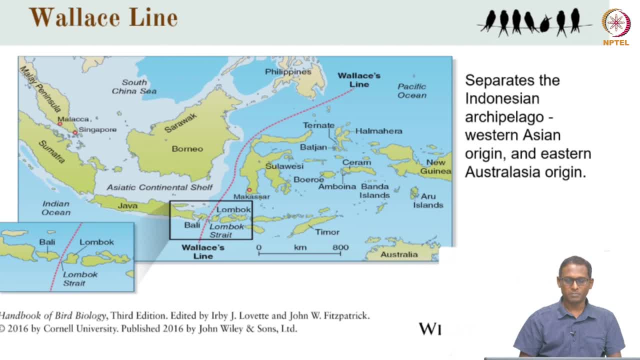 Asia. he was particularly impressed by the distributions that suddenly changed at some point. So he was out exploring different islands, But between Bali and Lombok, which are shown here, suddenly, which is in this area, suddenly he found that you know the distribution of species. 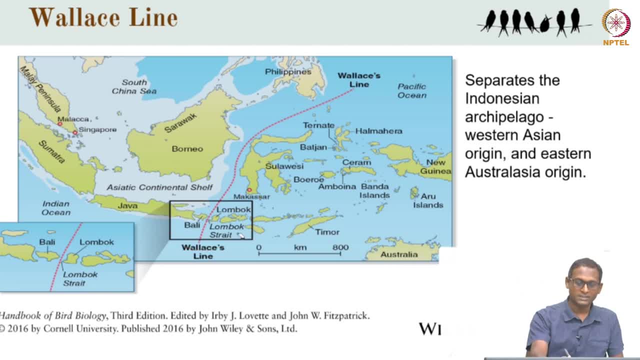 changed And he, after much investigation and thought, he proposed that a lot of the species in the Western side had an Asian origin and the Eastern had an Australasian origin. And What was surprising at that point was the line was very, very sharp and this area that 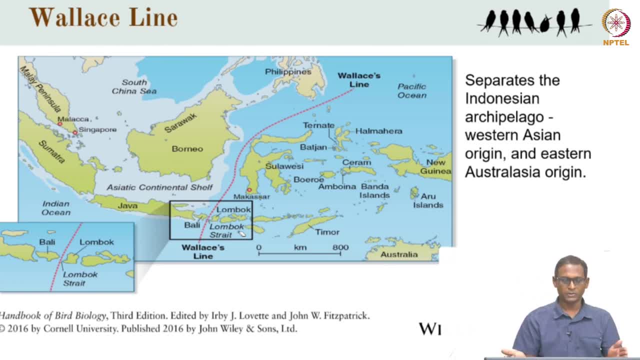 divides the two types of species distributions, is later been described as Wallace line and is important biogeographic barrier. It is recognized as an important biogeographic barrier. So what that means is that species that are from Australia, Australasia do not kind of 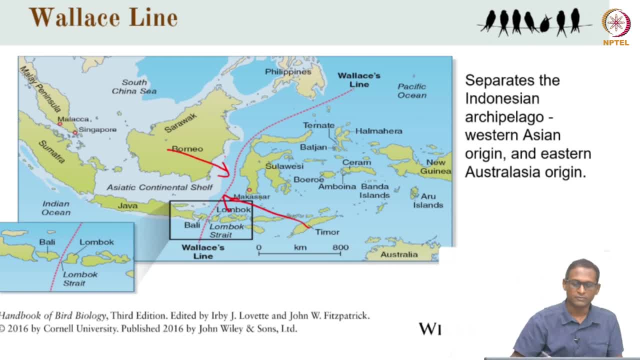 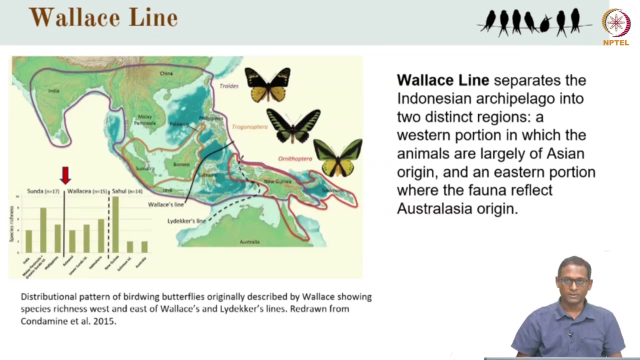 cross this and the others kind of you know. So this is like a distribution barrier for multiple species and that is what becomes a biogeographical barrier. This a very good example of Wallace line, and this biogeographical barrier is the distribution of these butterflies, these birdwing butterflies, and, as you can see there, 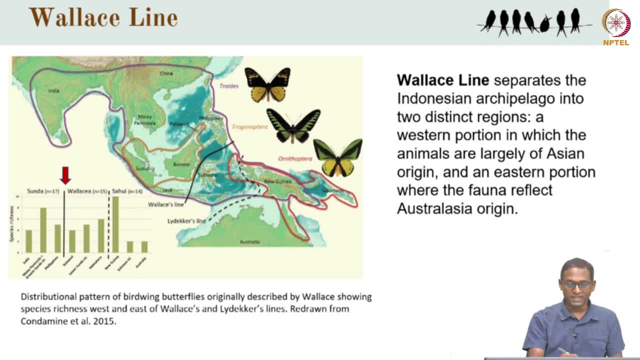 are different groups that are found only on the east or on the west of this line. So this was later revised and there is another biogeographic barrier like the one that is shown in the dotted lines here and that kind of shows how there are these very narrow areas. 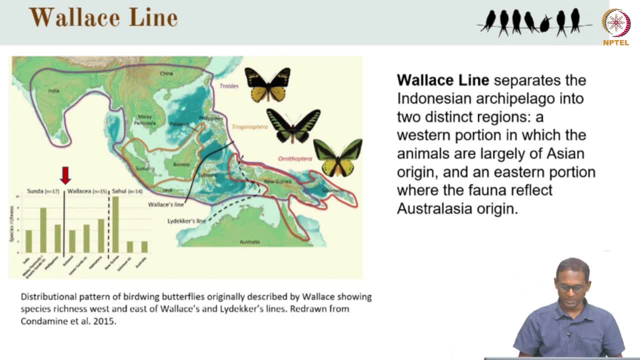 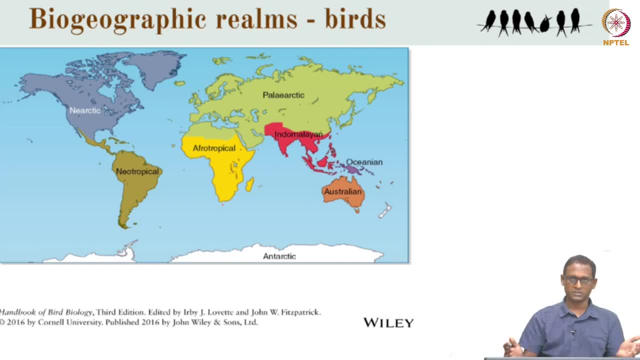 where, Where the species distributions change, and those are called biogeographic barriers. Now, based on similar biogeographic barriers all across the world, more recent studies have shown that there are. there are some areas that have distinct species distributions. One of them is where we are, is the Indo-Malayan region in the red. then you have the Paleoarctic. 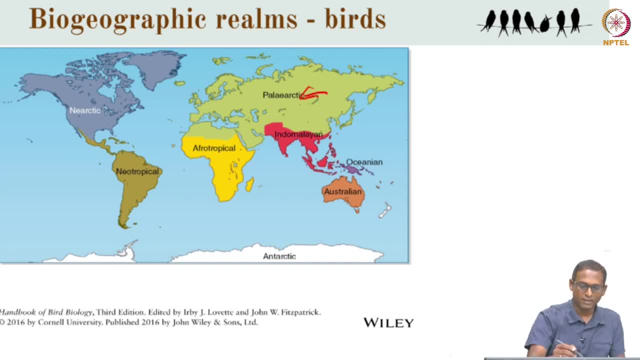 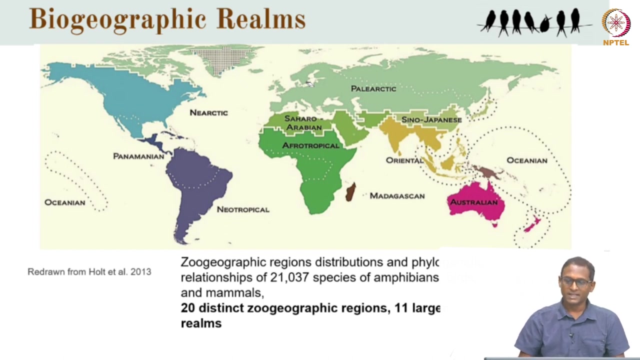 which is further north over here, And Afrotropical, Neotropical, Neartic and so on. So these are. these are the rough biogeographic barriers when you look at species distributions at a very global, large scale perspective. Other researchers, such as Holt et al in 2013, have refined and that they have other proposals as well. 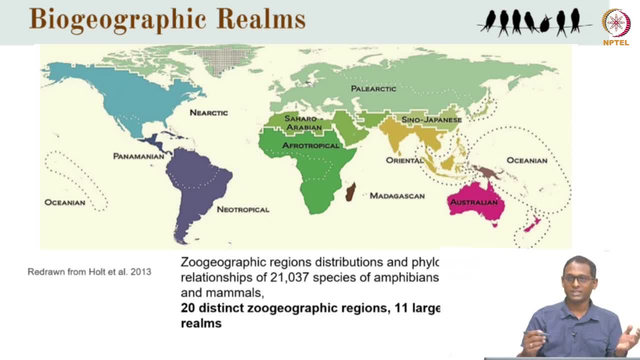 They have actually divided all of the species distributions. They have actually divided all of the species distributions. They have actually divided all of the species distributions, All of the area in the world into 20 zoo geographic regions and which they kind of club together to form 11 realms. and those are the ones that you can see here and you will notice that. 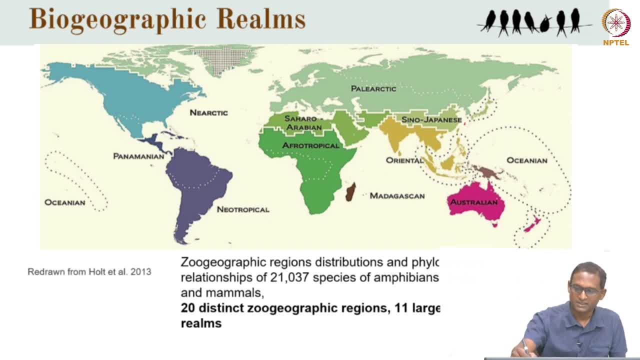 there is a new Sino-Japanese which has come here, yeah, But we are still in the oriental realm, which kind of you know makes that is kind of clubbed together. So these were made by examining the distribution of about 21 thousand species of amphibian's, birds and mammals. 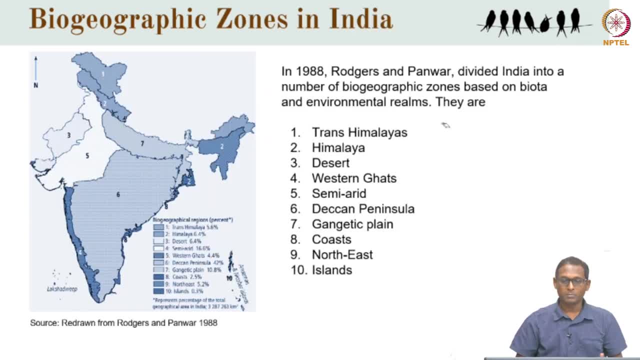 So it is not just birds. But what about biogeographic zones in India? just because we form part of the oriental realm, does that mean that we have unique- I mean just uniform diversity all across? No, that is not the case. In fact, there was a very monumental description of biogeography. 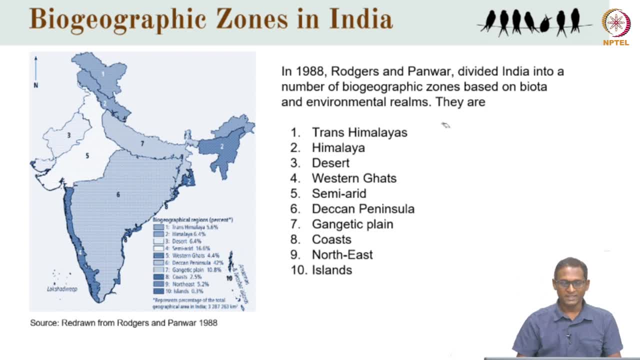 of India by Rogers and Pawar, and that was in 1988, was published in 1988 and they proposed various biogeographic areas which are still used even for conservation planning today, and in this you can see the list of the different areas. There is Trans-Himalayas, Himalaya. 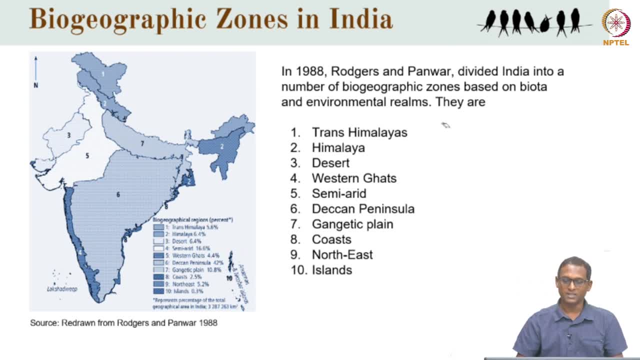 there is desert, there is Western Ghats, semi-arid, Deccan Plateau, Gangetic Plain coast northeast, and also the islands like the Narcondam, Andaman and Nicobar Island and the Lakshadweep Islands. 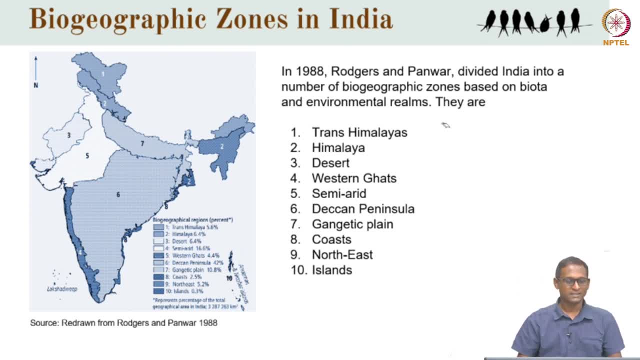 But you will still notice that there are some very missing aspects. For example, there are no Eastern Ghats. So if you are from anywhere near that, you would immediately say where are the Eastern Ghats? So you have to remember that these are very broad biogeographic barriers. 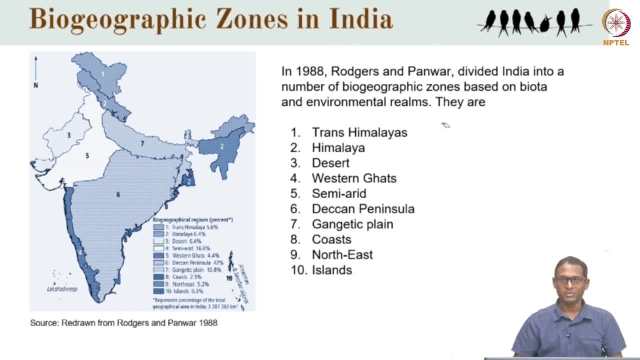 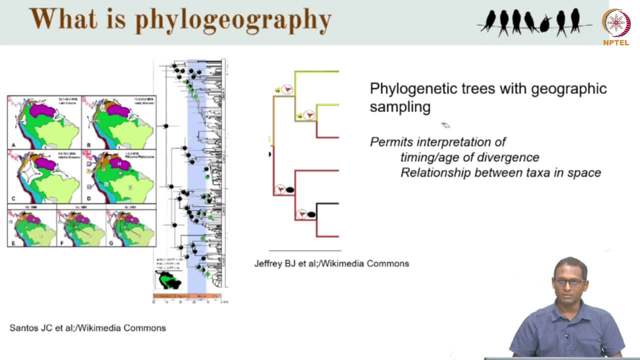 Within each of this you may find further divisions in biogeography, and how do people kind of come up with these ideas of distributions or biogeographic areas? So today people understand the biogeographic barriers and biogeographic divides using something called phylogeography. 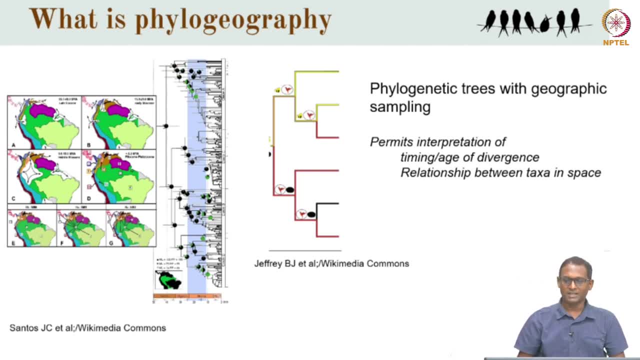 and I will explain what phylogeography is. At the heart of phylogeography are these phylogenetic trees, which is what you see here. This is relationships between organisms based on genetic data. Now, how this actually happens is that researchers go out and they collect genetic. 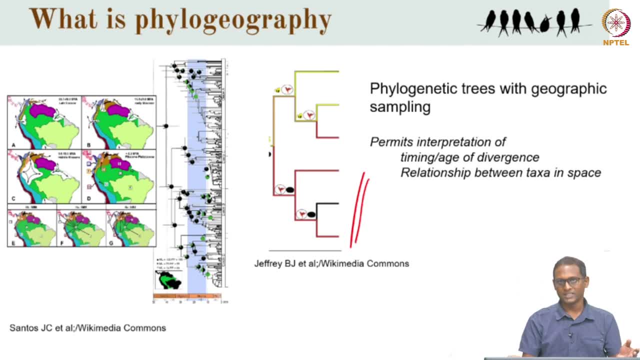 data from samples across themselves And they collect a collection of genetic data. And the researchers collect genetic data from wild animals, So they collect genetic data across a geographical space. For example, the authors here have on: the example that you see here on the left is poison frogs which are sampled from across South America and 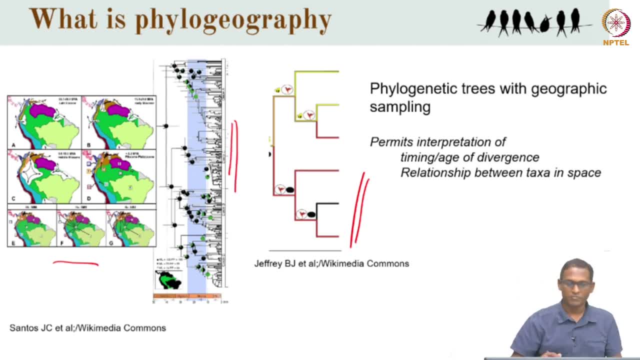 this results in this very complex tree that you can see here, which you do not have to really understand. But the point is that with such a tree with geographical sampling, they are able to estimate where species originate from, and in this case they find that the northern 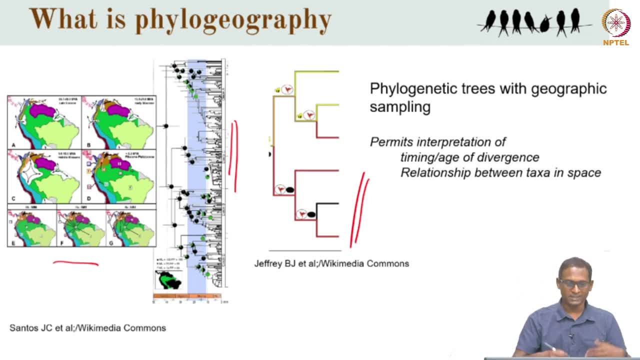 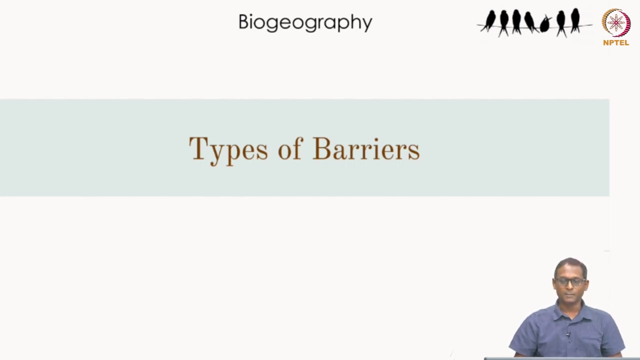 areas are where these poison frogs originated and then they moved southward from there. So essentially, what it what it helps us is understanding timing and age of divergence, and it helps us understand the relationship between taxa in space. Now that comes. That brings us to this question about barriers, because at every biogeographic point of turnover, 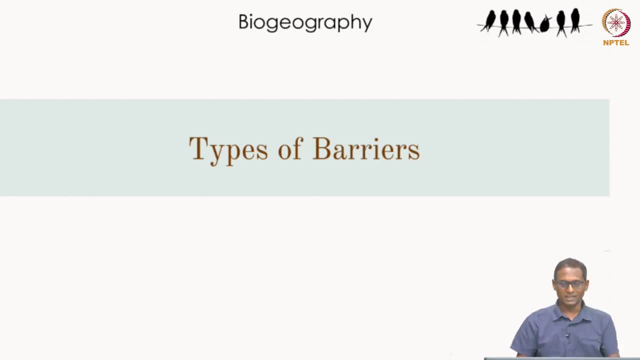 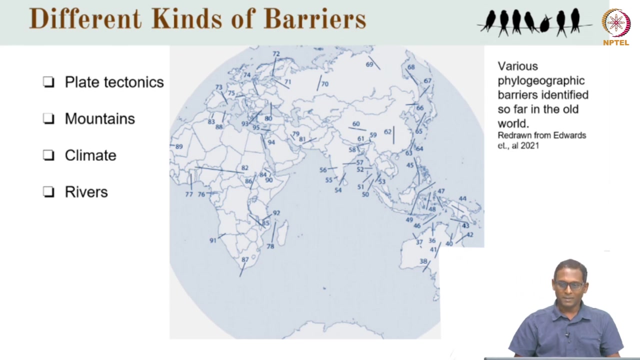 is a barrier and there are different kinds of barriers, and that really depends on what kinds of species we are talking about and what the nature of the barrier is, and we will discuss this in detail. So here is a map of A global distribution of various barriers that have been identified by colleagues Edwards. 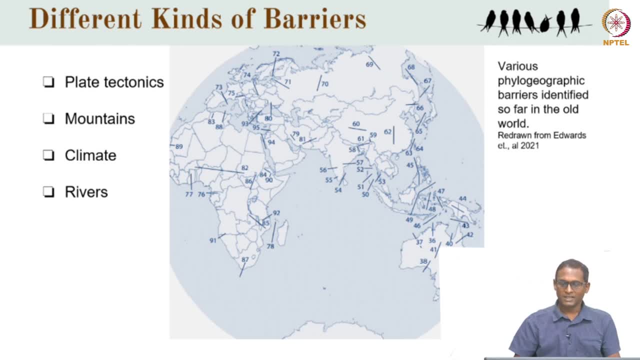 myself and few others, and essentially this shows a few potential barriers. This is still not exhaustive and what you know? what are the major drivers? sometimes it can be plate tectonics, and I will explain what that is. It can be Mountains, it can be climate, climatic differences, or it can be major big rivers, and we will. 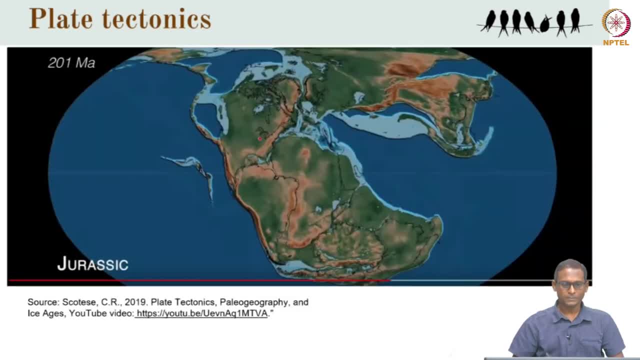 deal with each of these separately. So plate tectonics: I think that many of you would have you know, read somewhere or the other about plate tectonics, but just to bring everyone up to speed, I will play you this video, which is created from a lot of careful data. 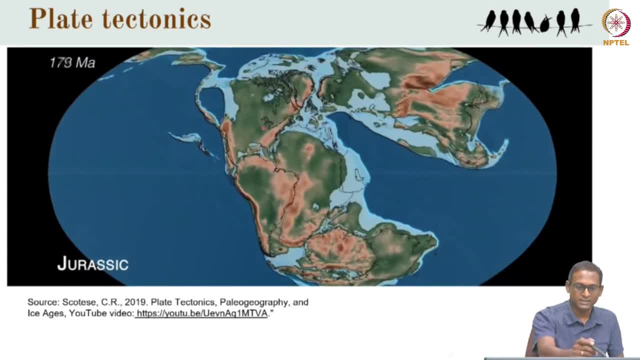 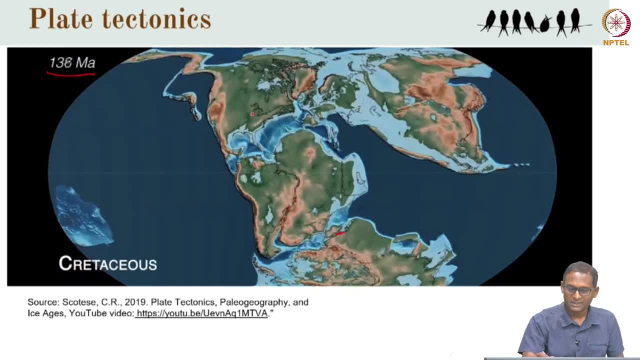 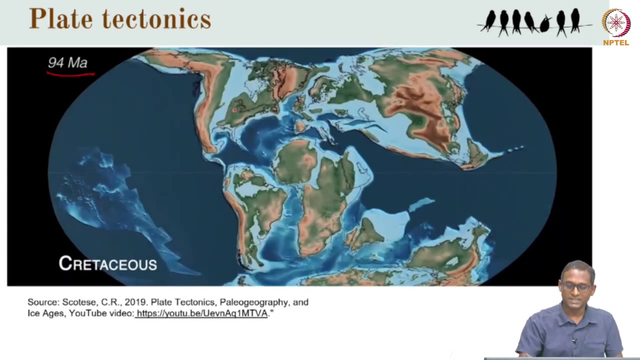 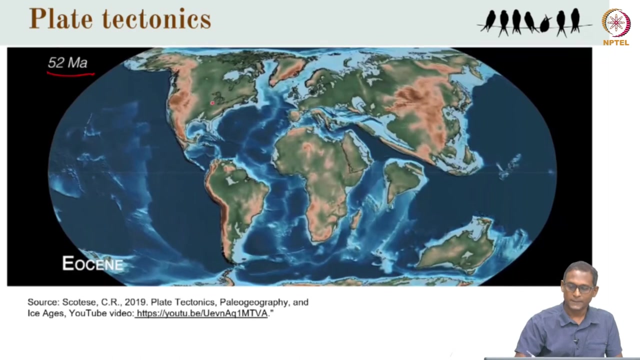 So this is in the Jurassic. you can see the time running here and you can see that India, Indian landmass is here and that kind of splits From the Pangea and, as follow the years, it splits from Madagascar And then it it crashes with the 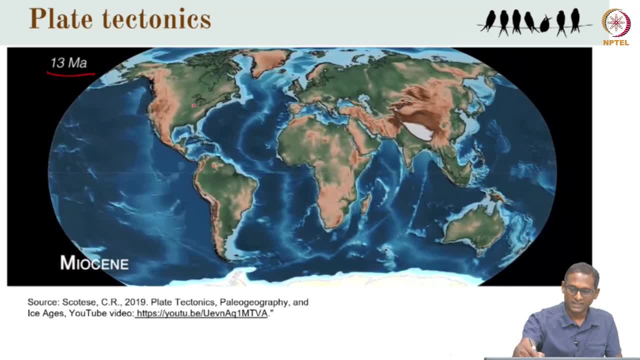 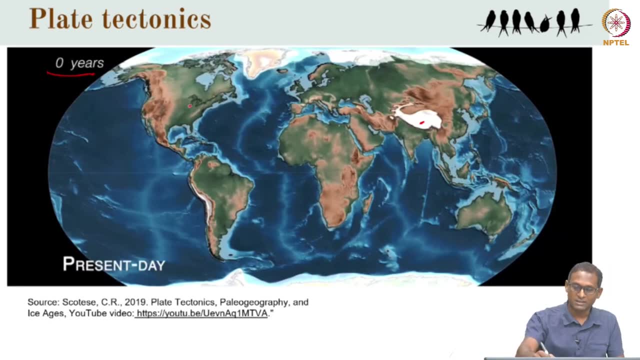 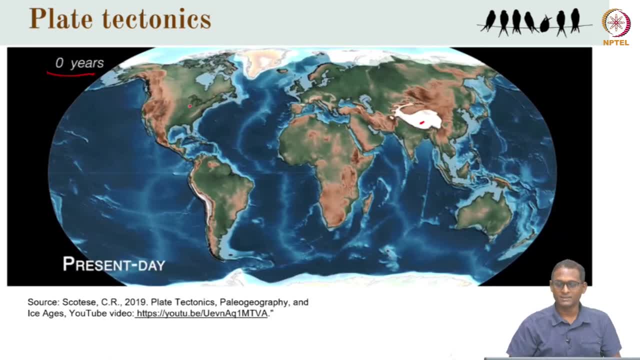 means that if some of these areas could be connected when the sea levels go down, Yeah, So now the point is that at some point some of these land masses were connected and then they later separated, So So. So if you had organisms that were on a particular landmass, there is a chance that that could. 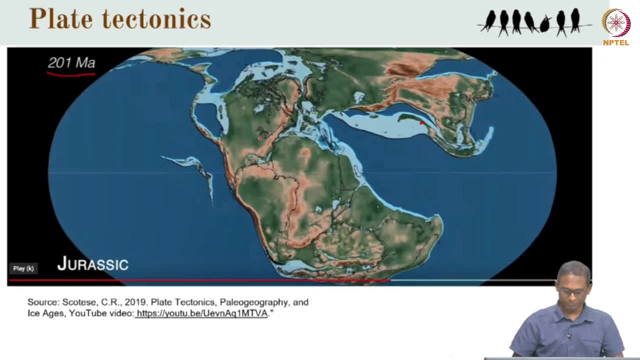 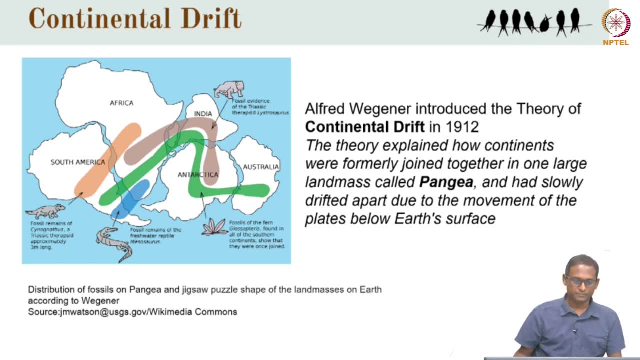 have kind of moved along with these continents, and this is- this idea is called continental drift. So here is a very nice representation of what continental drift could look like. So there are some fossil evidences of some Triassic species here and you can see how. 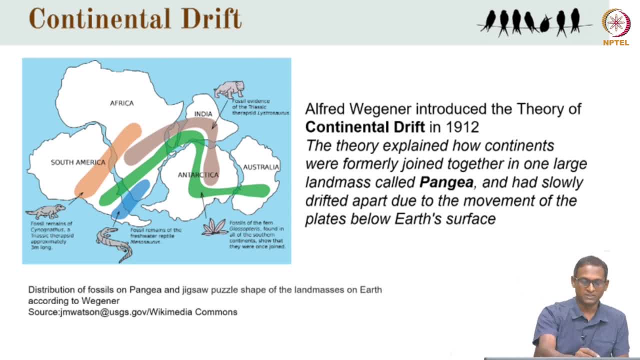 these connections run between continents. for example, some are found only in South America and Africa, but some others are found in Africa, Madagascar, India and even Antarctica and some others across. you know all of these continents And that is how people initially tried to kind of you know they were trying to understand. 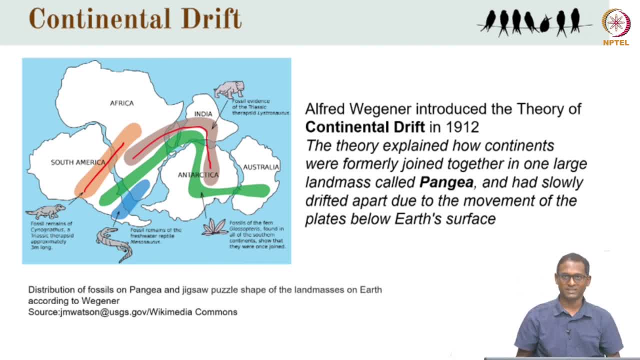 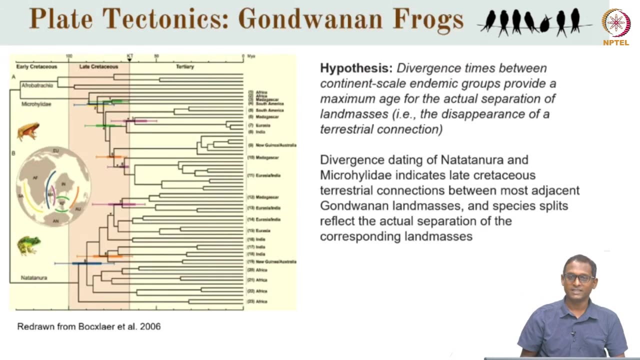 how Continents or how did these species get to these areas? and slowly, with data on the geology coming into place, it was like a jigsaw puzzle and people put this data together. More recent data, especially of relevance to India, are these ideas of frogs that have been 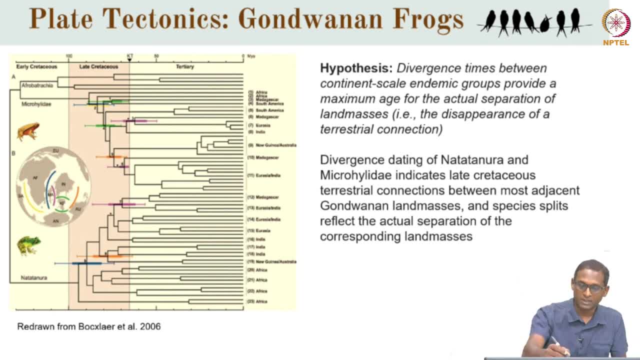 isolated from Madagascar for a very long time, For example. So you will. you will note that the Indian taxa are here and some are here, and the how to read this. this is a phylogenetic tree and on the axis that you see here are is the. 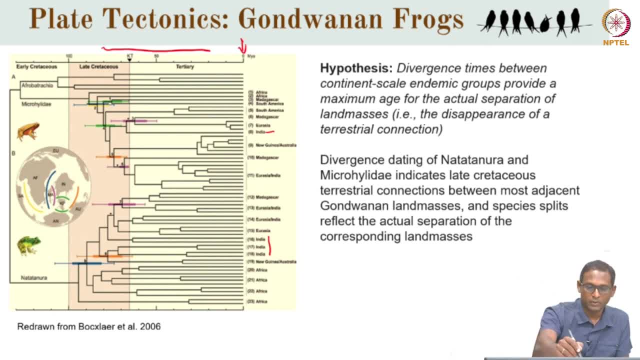 time. So, which means that we are here at 0 time point and as you go back in this direction, that is, you know, in the past. So this means that about 100 million years ago there was, You know, These two groups had split and then later on at the KT, when the KT extinction happened. 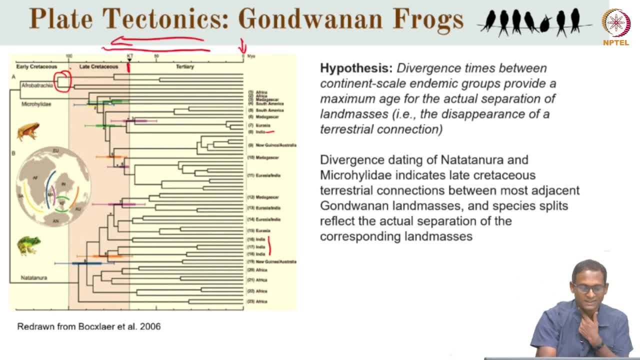 that was around this time and if you follow this line, that is when all of these species had split And you will notice that several of the Indian species split from the other areas around. you know, around the time that people describe the, you know the plate tectonics. 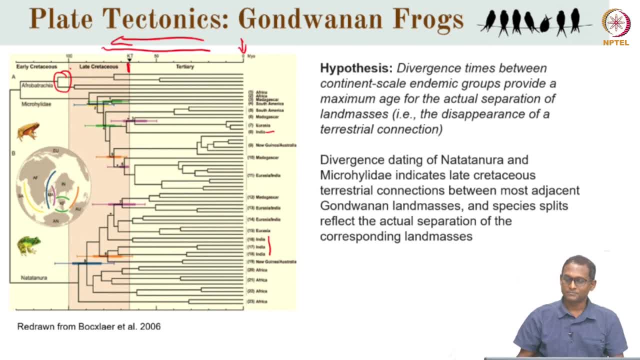 So some of these dates coincide and so this has been a hypothesis- how people have used genetic data along with fossils to calibrate and get ages of the timing of divergences of different taxa and how that relates to the geology of these land masses. 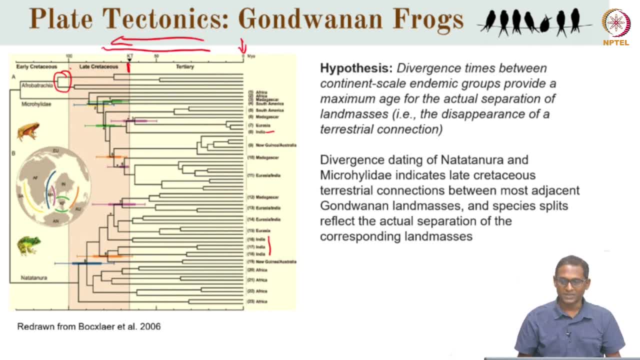 So this is really fascinating. more and more data is coming out, So this is a very interesting part of our discussion, and I hope that you are enjoying this research. Now for the next few minutes, I would like to take some of your questions and then I 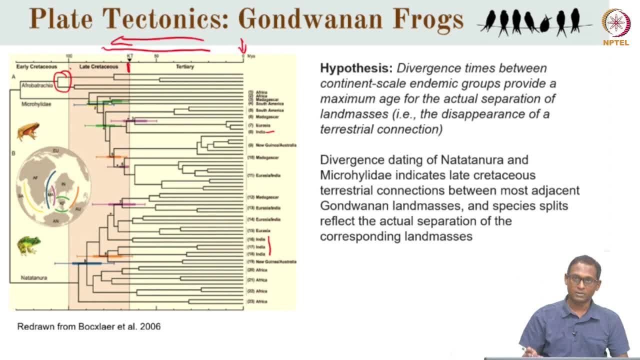 will get back to the discussion on the next two points. So if you want to follow these two points as you go on with your questions, we will have time for some of the questions from the audience. So let us now continue with the questions that we have received from our audience. 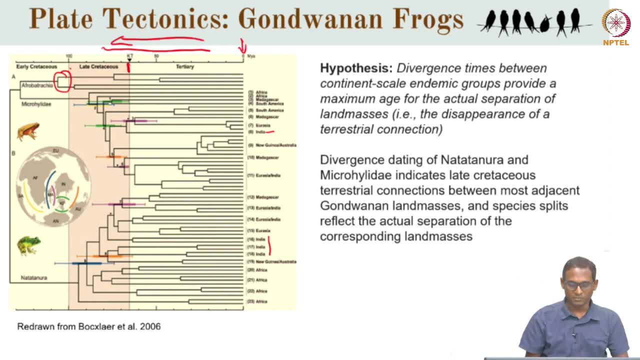 So for the next few minutes, I would like to take some of the questions from our audience. so please feel free to pose your questions and let us go through them. I will be taking questions from the audience. So the first question is: what is the relationship between the two species and the species? 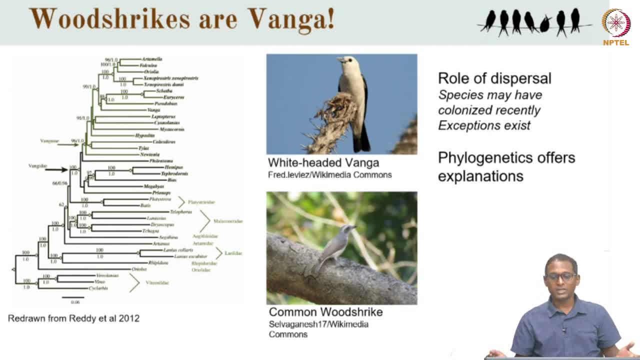 Now I will be studying the species of the species. So the species of the species is a very specific species and it is an extremely complex species. So, but, however, not everything needs to be with. you know, dispersal due to continental drift. 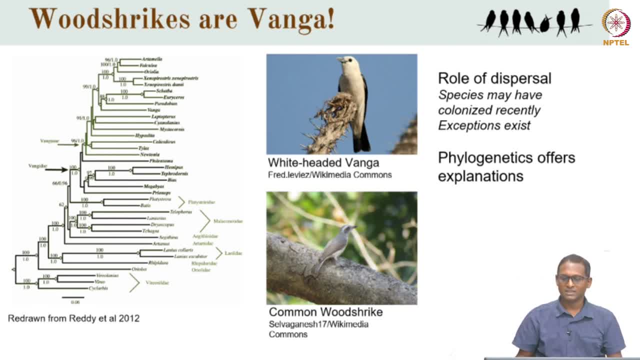 it can all. there are also exceptions, For example, this bird that I think many of you may have seen in India, the common wood shrike. actually, it turns out that it is not. it is not a taxa that is related to other wood shrikes, but it is actually related to vanga. these groups of 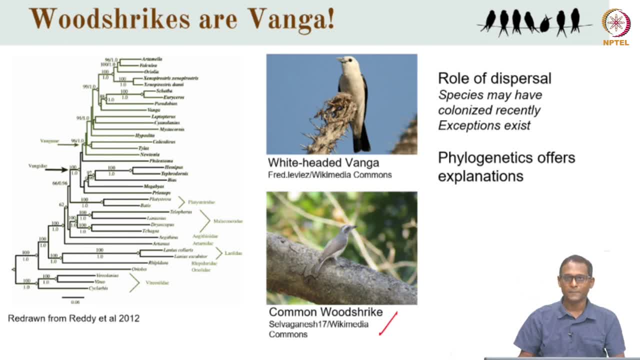 birds in Madagascar, and this was a fascinating paper by Sushma Reddy's group where they showed that some of these species are. they might have actually moved across from Madagascar to India, So this is not very old. that is a important point that I am trying to make. this is not a continental 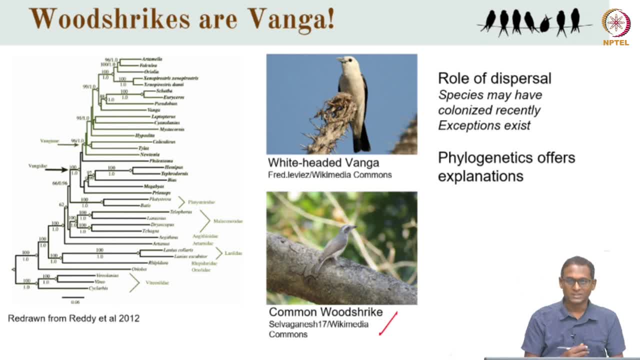 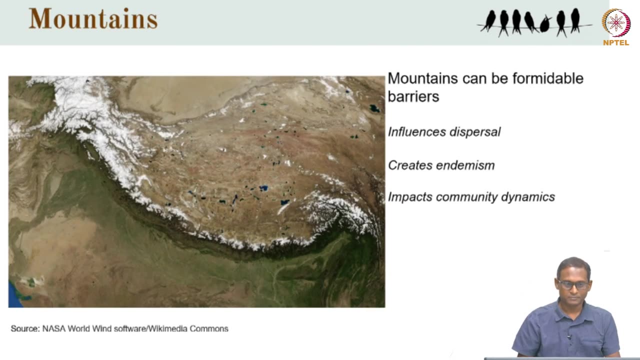 drift example. it is a more recent dispersal through maybe jumping across oceanic islands and so on, But those are all hypotheses. but the fact remains that the common wood shrike is actually a vanga. So that is. that was all about the plate tectonics and some exceptions. 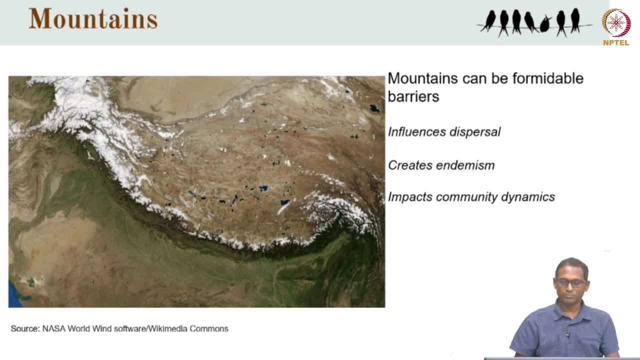 We will now come to the other barrier, which is mountains, and mountains are actually formidable. they are, of course, in different continents, different parts of the world and they can become formidable barriers because it influences dispersal. So some species are not able to move and cross across these barriers. 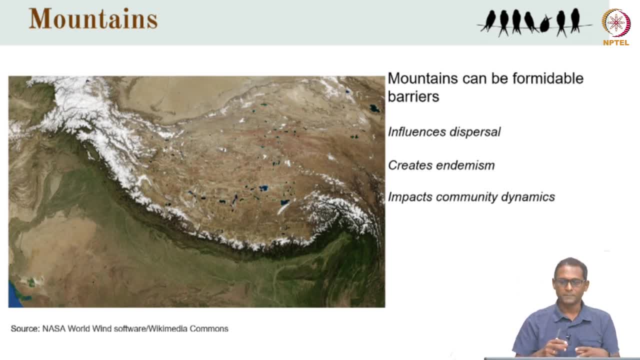 and it can sometimes create some kind of endemism, which means that some species are restricted only to certain mountains- We will talk about a few examples here- and it can impact community communities and community dynamics, and we will have some examples on that as well. 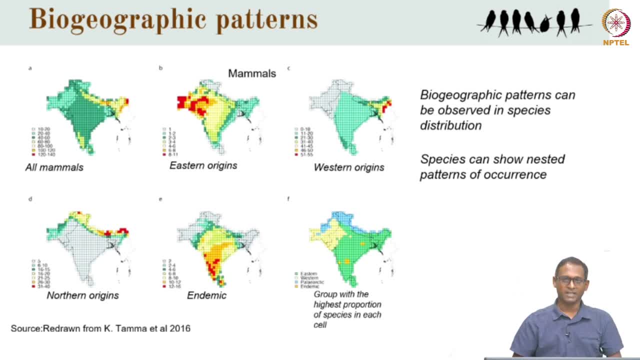 When we start with that. in a fascinating study by Tamman et al in 2016, they showed how different biogeographic patterns can be seen in mammals. For example, not all mammals show similar biodiversity patterns in this various maps that you see. The first one here is for all mammals. Essentially, it says: if you grid up India. 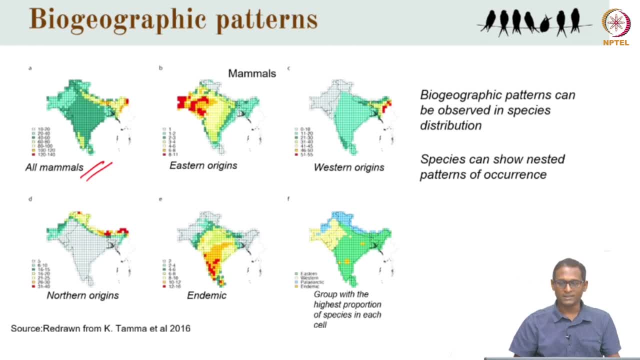 where does this? exists Even India, where some animal did not go. What you see it, this area? as where do you, in which grids do you find most of the mammals? And yes, you find more of them in the northeast and then some here and so on, But then this seems to be hiding some patterns. 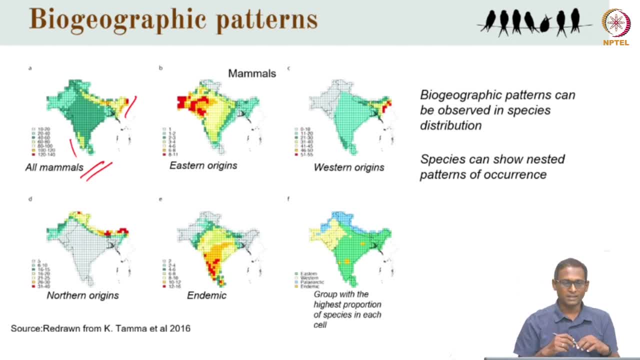 If you start looking for species that have eastern origins, which means that they are from the Eastern Realm, somewhere you know, from afro, tropical or some other areas, So those are clearly more found in the eastern parts. Similarly, you have some with western origins. 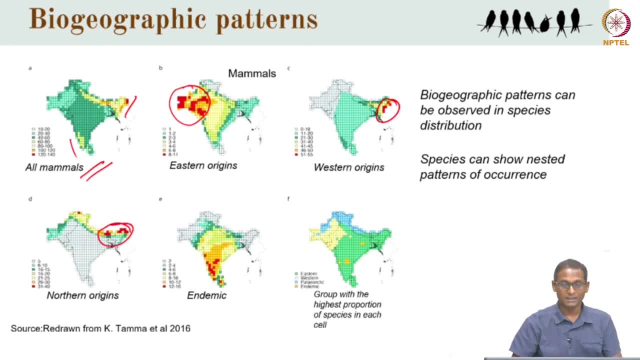 and some that are that have northern origins, and understandably so. You can see that some of them filter through and they are able to go further in inland right. well, this is not a very good example because, as you can see, most of the northern ones do. 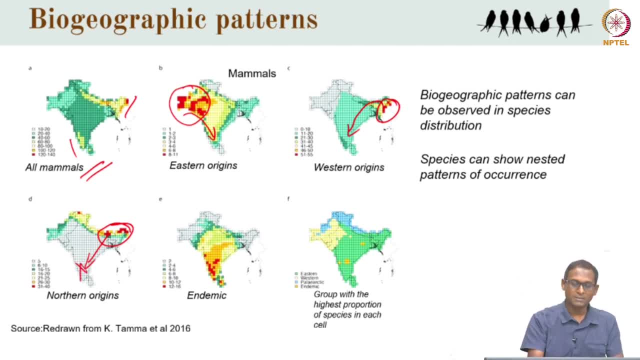 not make it further south. There are also some endemics, which means that they are largely found only in India and are not found anywhere else, and those are seem to be in the peninsula, along the western Ghats and some parts of the eastern the Deccan plateau as well. So 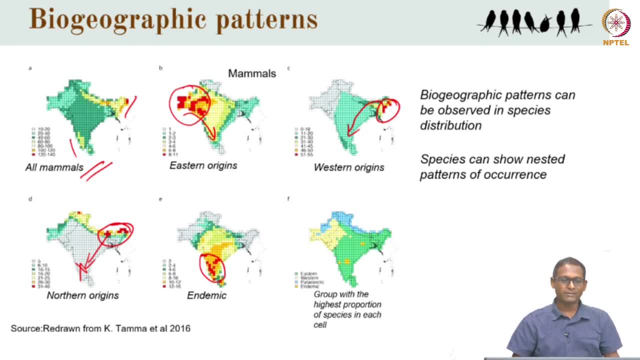 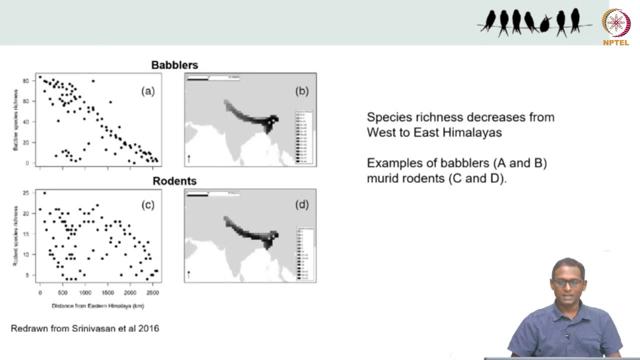 what this shows is that there may be patterns even within a specific area and for specific taxonomic groups. Another set of wonderful examples are on birds, from Umesh Srinivasan and co-authors, and here what they show is that a lot, not just, you know, babblers that. 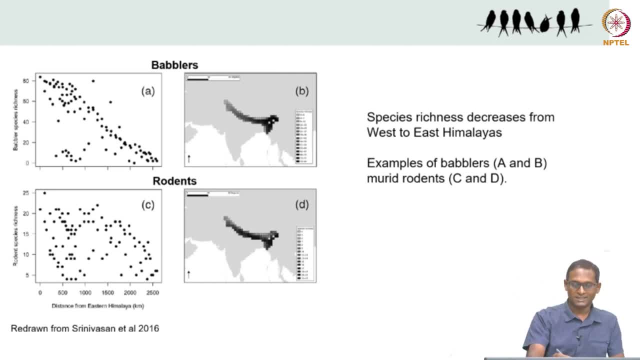 they focused on, but also murid rodents. As you can see in this picture, you can see that they are not only in the western Ghats. as you can see in this picture, you can see that they are not only in the western Ghats. 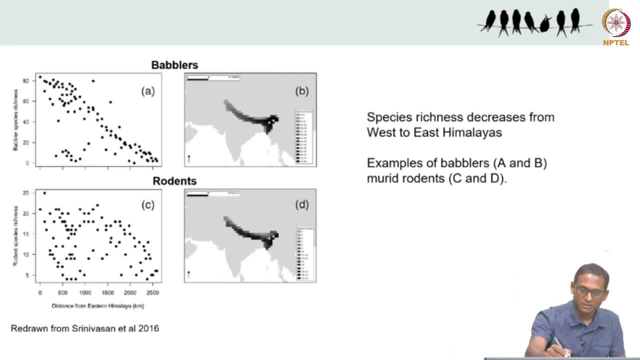 but when you go from the eastern part of the Himalayas towards the west, there is some kind of decrease in species richness and this they find in babblers and these murid rodents. So there is nestedness in distribution that they find. So it is very interesting to understand. 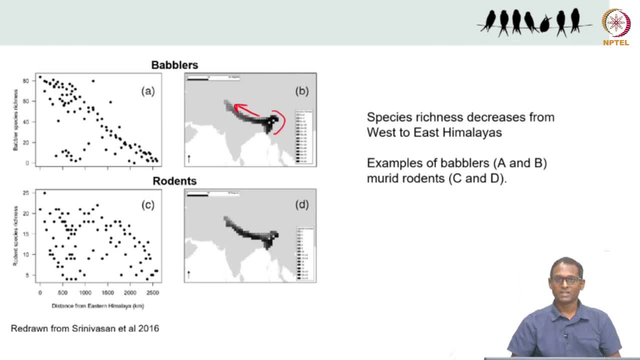 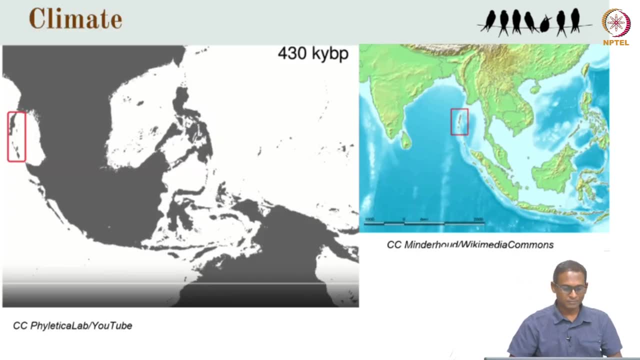 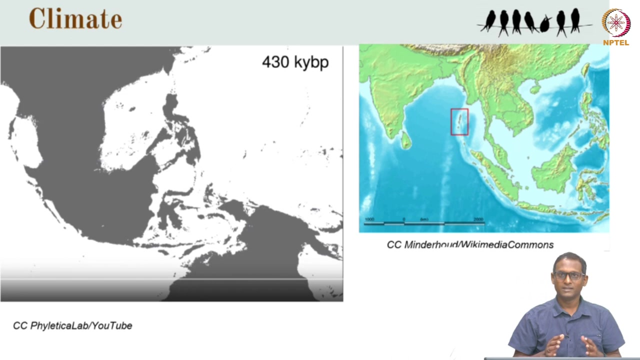 that the patterns of distributions of species can be understood by looking at distribution along each of those small grids. very fascinating. And here we like to move on to another aspect, which is climate, and for climate I would like to kind of take a moment to So climate can also be a barrier, but there are different. 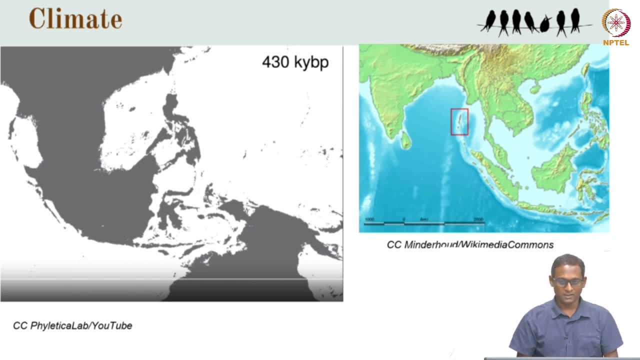 ways that climate acts on. So climate can also be a barrier, but there are different ways that climate acts on species and species distributions. I will start by first showing you a video of the Andaman-Nicobar islands. So this is the Andaman-Nicobar islands. actually, that is only the Andaman. 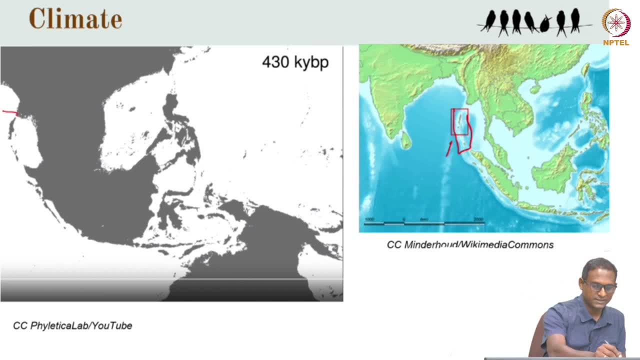 the Nicobar, go further down, and which is this area here? And what I want you to notice is how the how this area kind of changes, and I have a video here again from the, from a lab that has created this with data on how the ocean levels have varied through time. 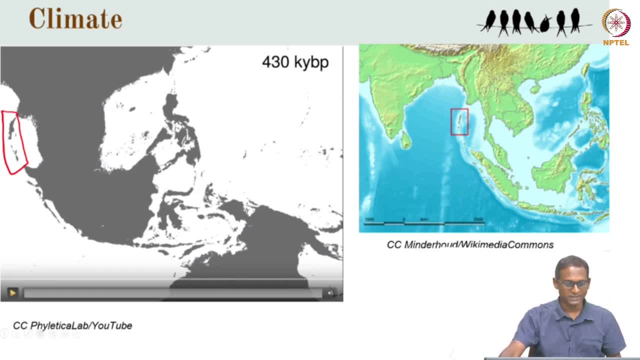 So we will start with 430,000 years back and you notice that the land was much closer, much closer to the sea level. So you can see that the land was much closer to the sea level. So you can see that the land was much closer to the sea level. So you can see that the 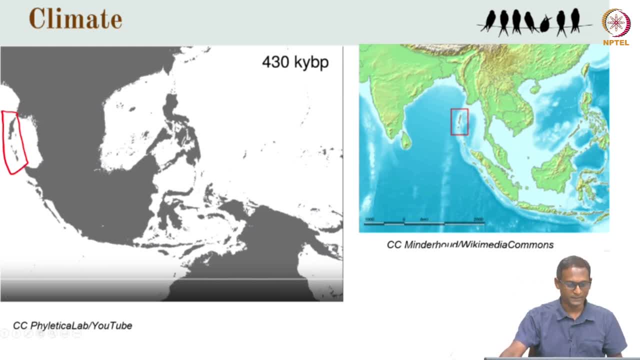 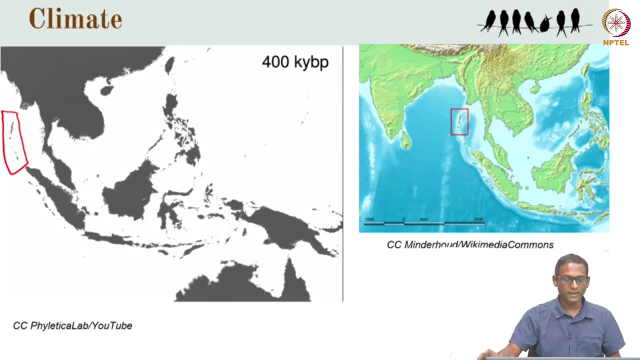 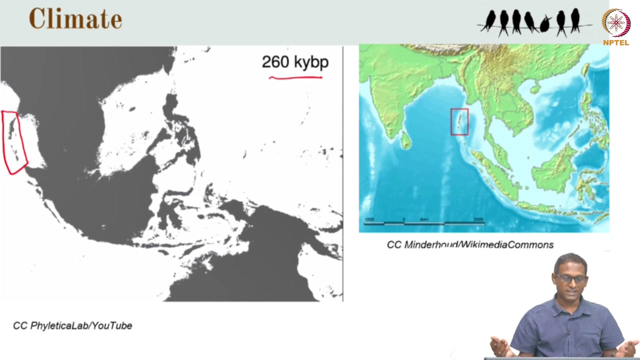 land was much closer to the sea level between Andaman s and the Mainland here And I am just going to start playing this video and you will see how the oceans kind of contract and expand through different points in time and time is here, So at some points they are very isolated and at some others the land. These are called. 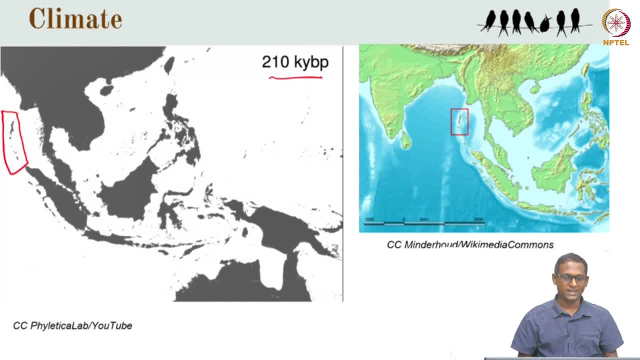 some kind of land bridges. There are some bridges formed and these bridges allow for species, various kinds of species, to cross across them, and this is colonization of some way or the other. So this is 70060, yeah, and this is our current scenario. 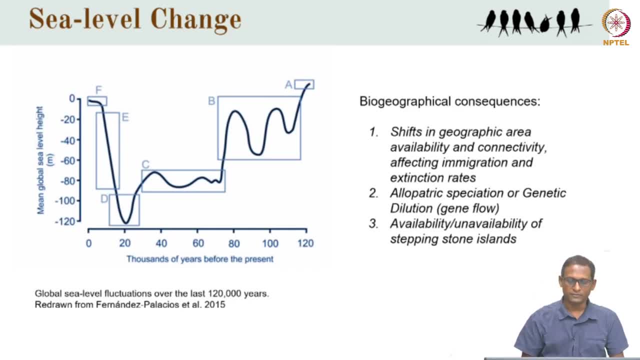 Sea level changes. so this is what we just saw an animation of, but you can also see, you can visualize this in different ways. you can think of time before present. this is in thousands of years, right, and as you can see that, as you know, at some point the global sea level, 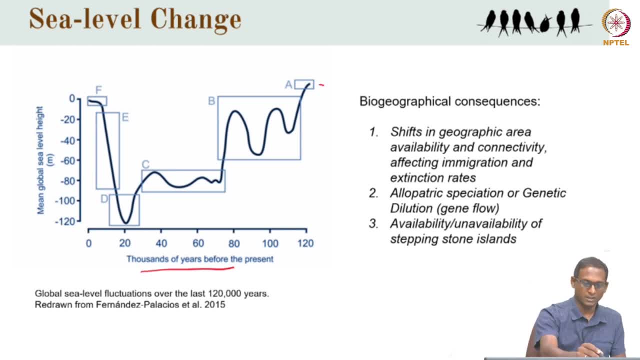 was here And although we are very close to that now which is here, It has gone through times when the sea level was different by even 120 meters, right So, and at 100, at that kind of time point. this is the LGM, the last glacial maxima, that is. 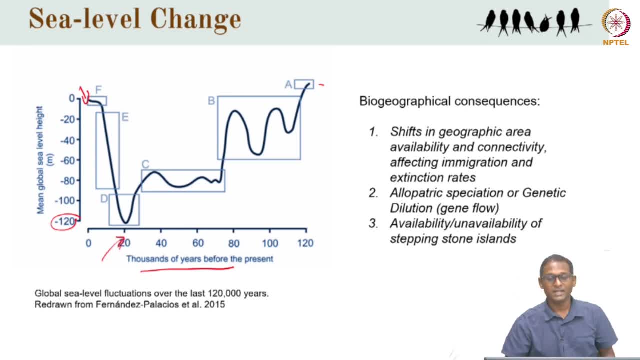 about 18, 20,000 years back And at that time point a lot of the sea level was much lower, permitting movement of organisms between Several areas connected by land. this was also time when there was a lot of aridity, which means that a lot of the wet habitats moved up the mountains, especially in the tropical. 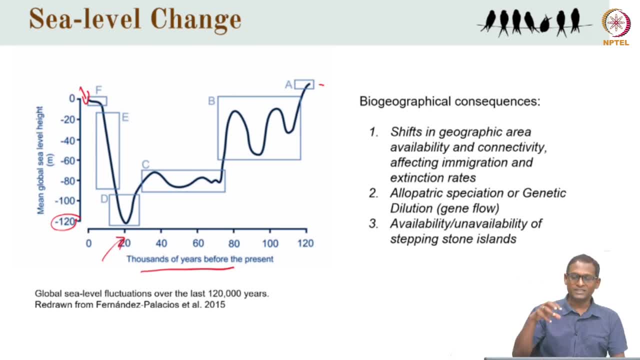 mountain systems. So you had only some areas on the tops of the mountains with some relict habitat, So we'll talk about that as well. So these these changes brought about a lot of allopratic, allopatric species Speciation and gene flow and created different levels of stepping stones of islands. 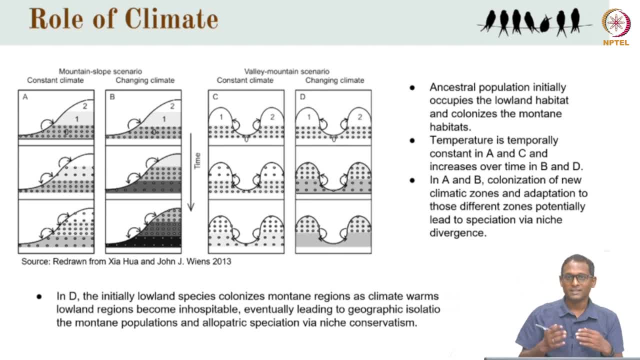 And mountains can obviously interconnect with the role of climate and this is very nicely illustrated by these different, by these authors who show a possibility of how species change, When, When, the different scenarios, the different possible scenarios: if, when, the climate is constant versus if it is a changing climate. 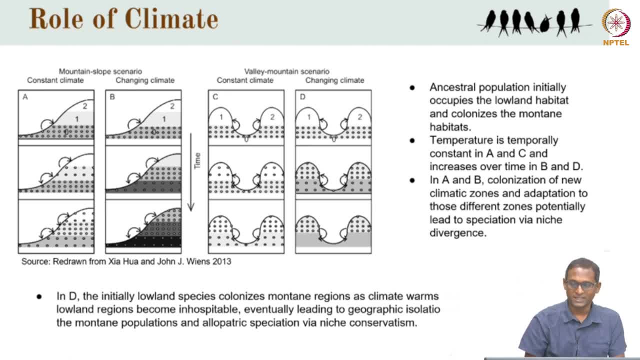 And so you have a mountain slope scenario and a valley mountain scenario And ancestral populations. initially they suppose they inhabit lowland habitat. they can colonize the upper mountains. So that is one of the one of the ideas. And And in some cases the temperature is constant, for example in A and C, and it increases in. 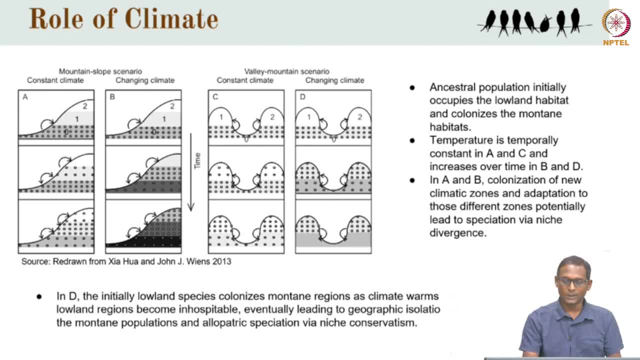 time over in B and D And you can see how this colonization changes and it can lead to speciation by niche divergence. And niche divergence is when they kind of occupy, they use different ecological aspects. that is, species use different ecological aspects. This Is 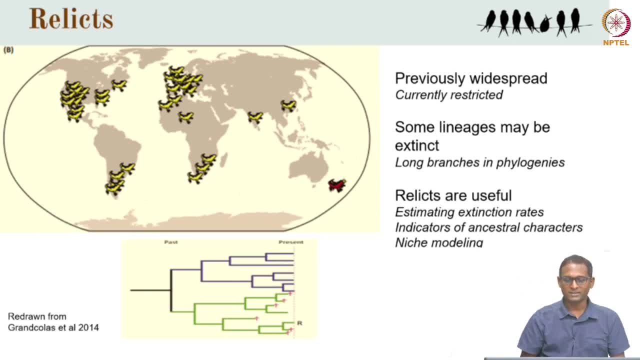 This is an example of relics. You can imagine a species which was found all across the globe, But what? what happens is that they go extinct. Some of the lineages go extinct and you can study these such relics by using phylogenies, For example. this phylogeny here shows that if you look at current taxa, it shows only 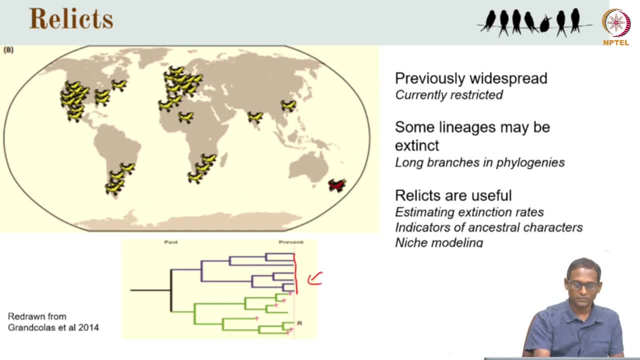 these purple ones, And so all of these have kind of gone extinct. and here is one kind of relic, relic species that is there In this example. you can imagine a relic on this on these island where they have gone extinct from all over the world. 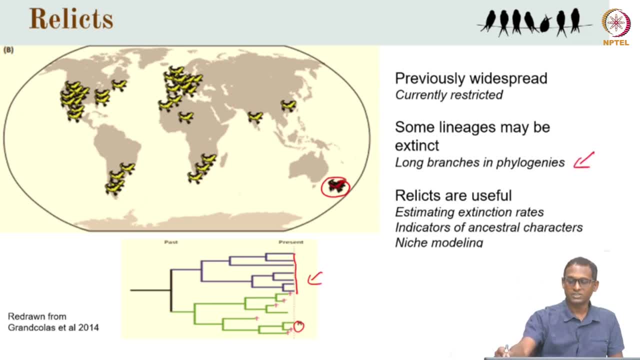 So relics are. they usually have long branches in the phylogenies and one must not assume that You know, That is the only diversity that is there today. that is what you see today because of extinction that has happened in the past. So it is useful for understanding extinction rates. 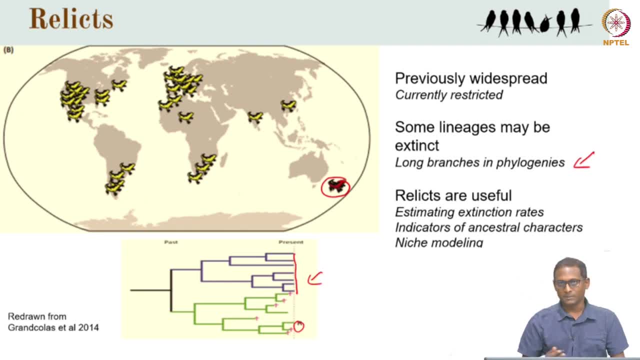 They are indicators of ancestral characters. for example, this fossorial frog that has some kind of a Gondwanan origin- the purple frog, you know it, that is very. that is a good indicator of All ancestral characters like this is a burrowing frog that comes out very rarely and it seems 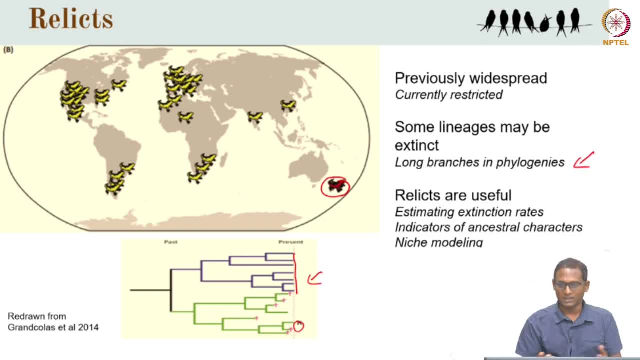 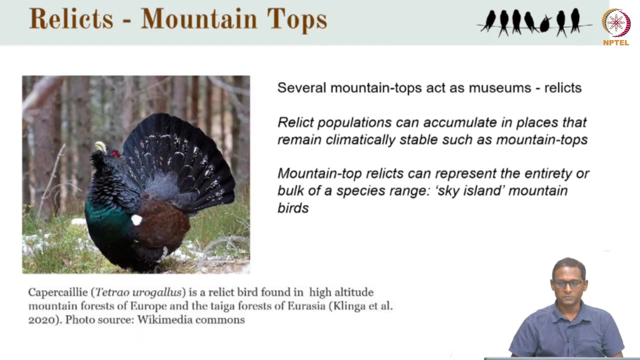 to have survived several of these climatic changes that have happened through in the earth through this period. One can look at how the niche has changed with niche modeling studies as well. Relics on are also found on mountain tops, so several mountain tops, the tops of the mountains. 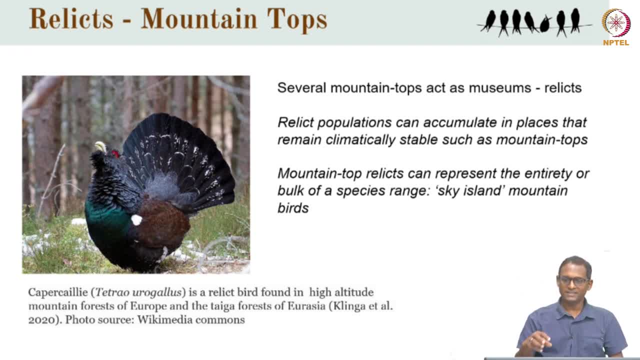 Host Different kind of habitat and these, these mountain tops can act as museums, where these relic species tend to accumulate, and that is largely because these mountain tops tend to be climatically stable. so, while the climate changes drastically in the lower elevations, on the tops of the mountains, because of humidity and temperature differences, the climate tends. 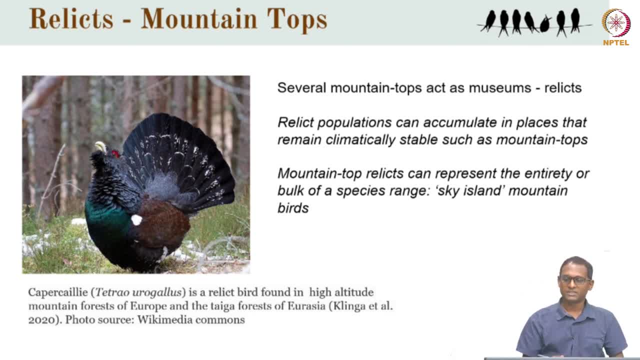 to remain more stable. And these mountain tops: if you have a series of mountain, they become a series of these museums, and these are. these are called sky islands because the habitats are found isolated from each other, and this here is an example of a relic bird which is found in the high 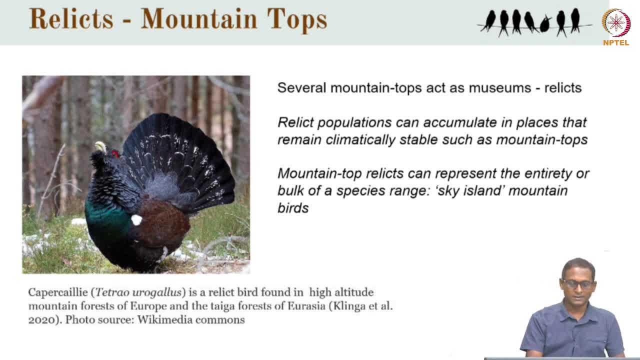 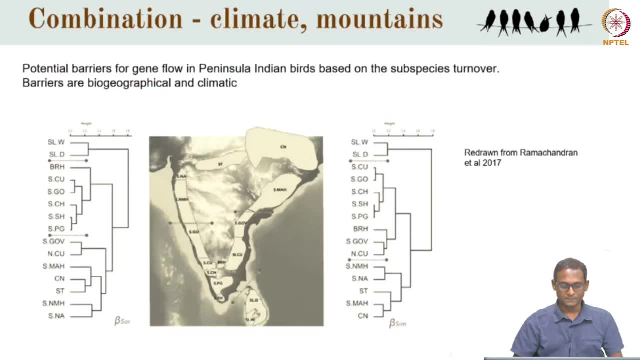 altitude mountains of Europe. yeah, So, So, So you can find. there are other examples that we will come to, even in, even in India. So what can also happen is that it's not climate or mountain that act independently. in some cases, people are not able to differentiate between these barriers, because you may have 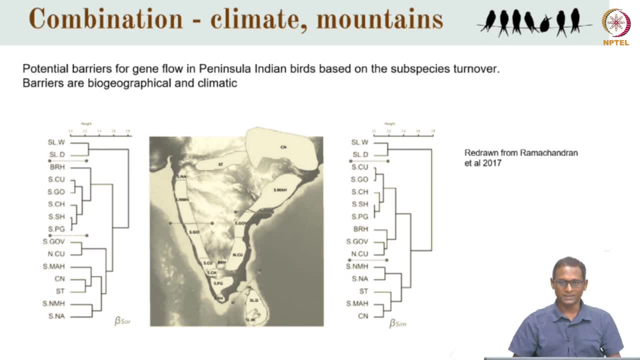 a climatic barrier and geographical barrier, a mountain barrier, So So, So in this study, let just to kind of keep you focused, if you, if you consider the diagram here, the map, there are these lines. So these are three areas where these authors, Ramachandran et al, which included me also. 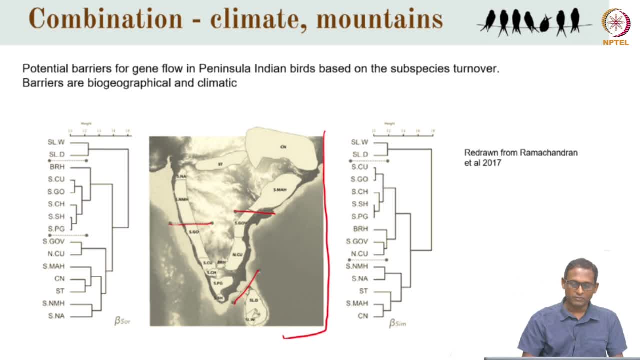 looked at bird distributions and what we found was that the major barriers, major locations of turnover of subspecies- this was based on subspecies, it is not based on genetic data. So these were the areas where there was a lot of turnover and you will note that there. 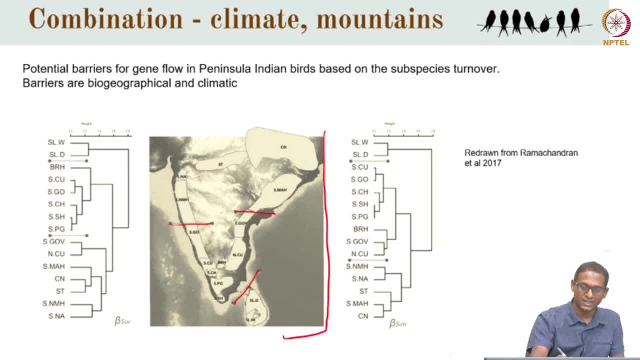 are several other minor areas which do not have these lines. So all the areas with the red line are the ones with which are major barriers in turnover of species. So, So, So, these you know lines that you see the dots those are. those are more minor areas of turnover. 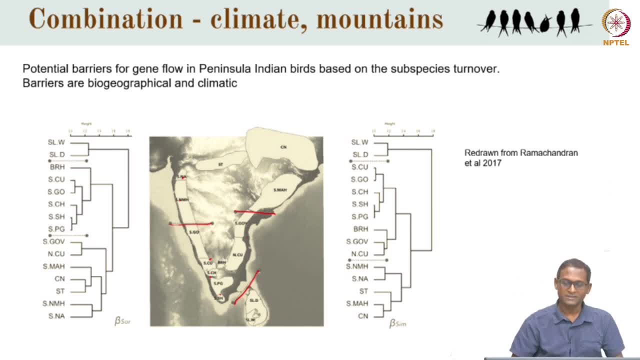 of species, of subspecies. Now, what this means is, if you go across, for example, the Palghat gap, which is here, there are several subspecies that are not found on the other side. you know, this is just like the Wallace line, And I am talking about only bird data here. 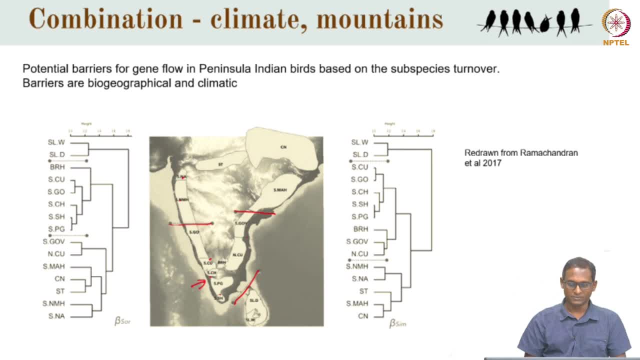 But I am sure that this is the case with several other species as well- And what they find is that, despite this, the major barriers happen to be the one here which is considered, or very popularly known, as the Goa gap, And that one appears to be more of a climatic barrier than a geographical barrier. 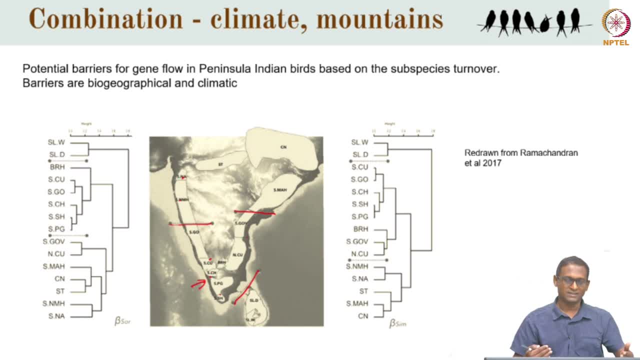 Yes, the Western Ghats are there, But there is no mountain pass, No geographical feature that you can identify with that barrier. So this is primarily a climatic barrier which has resulted in different vegetation structure in the north, different type of habitat compared to the south. 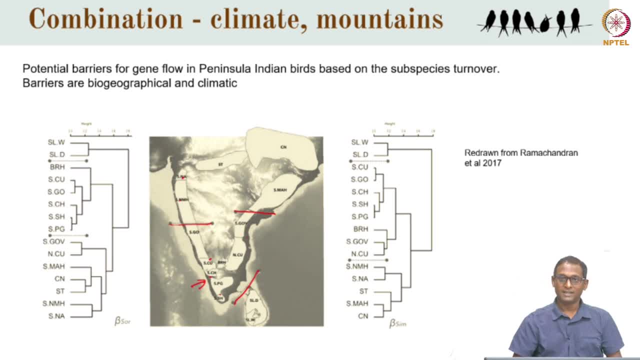 And the Godavari area here is a big river and it is kind of a paleo river. plus, there is a climatic difference, So it is very difficult to tease apart what is the role of climate versus a geographical barrier in some cases. But what is important for us to understand is that there are different kinds of barriers. 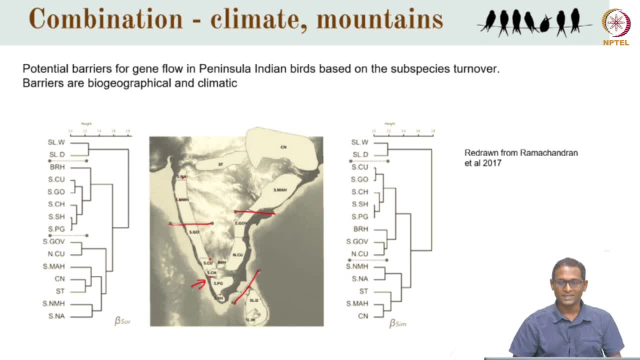 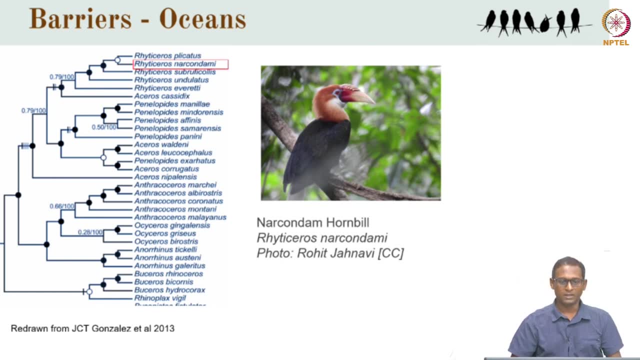 some of them are mountain barriers, some of them are climatic and some of them may act in combination, Going back to the barriers of oceanic on oceanic islands. I think Many of us know of this very famous example of Narcondam hornbill, the image that you see. 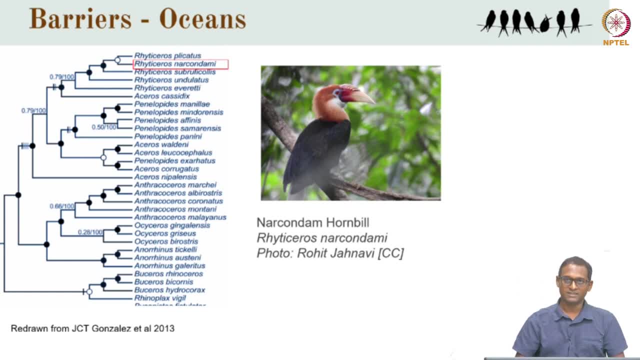 here, and this is. this population is found only on a single volcanic island called the Narcondam, which is where it gets the name from, But interestingly, the genetic data from 2013 seems to show that it is not very different from the other hornbill in the mainland. 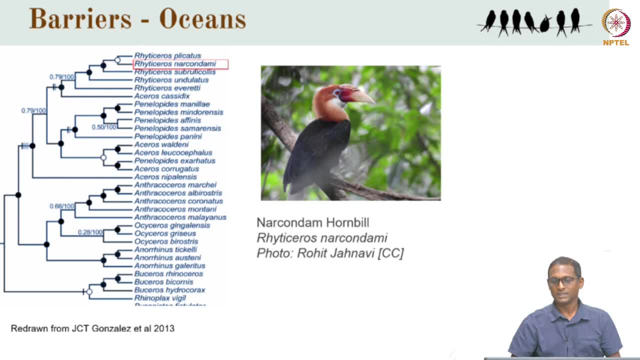 So this needs to be examined further, But the this may be because of how organisms can travel. if they are able to disperse across some of these barriers, then the gene flow is maintained and then they are not different species. So in this case, the there is no clear outcome so far. Yeah. 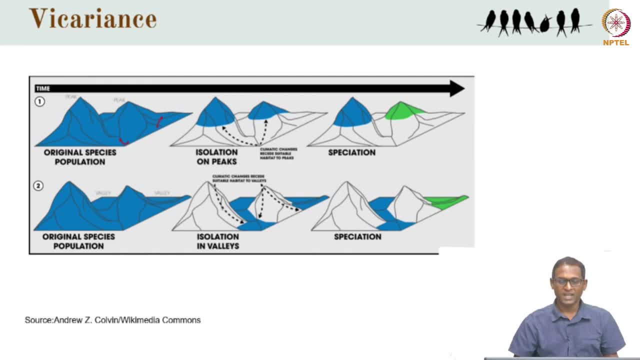 and the climate, let us say, changes, and there are two possibilities that can happen. One is that the species all move up. they go up the mountain and they get isolated on these mountain tops. this is one of the scenarios that we discussed earlier. In some cases, species may 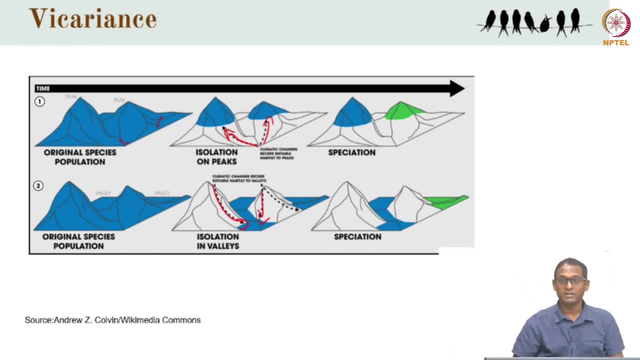 actually move down and even they are kind of tracking suitable habitat. that depends on where the you know what changes happen on these mountain tops, In some cases where there was some form of glaciation or ice formation when these mountain top became very cold, especially in the northern. 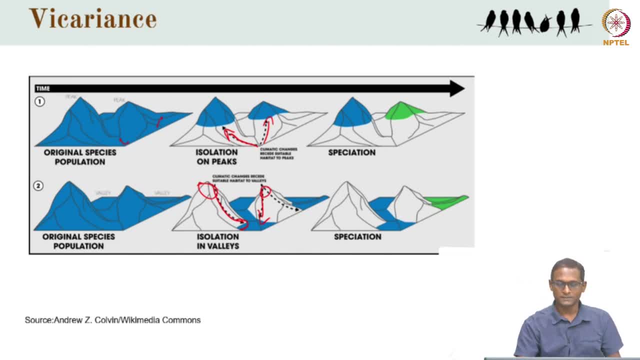 latitudes, they are known to go down into the valleys and over time. So as time goes by, it is possible that you can have a species a and species b just by genetic drift over very long periods of time. It is also possible that even the valley species can get isolated because of the mountain, So you 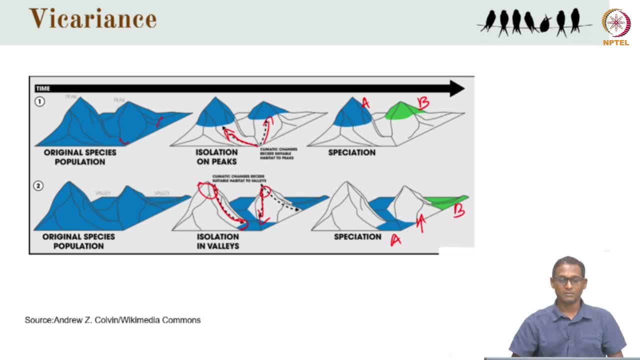 can have species a and species b here because of this. So the point here is that this kind of model of- of you know- speciation is called vicarians, and this is an important idea in biogeography. You can also have dispersal, where you have one species which kind of colonizes, moves. 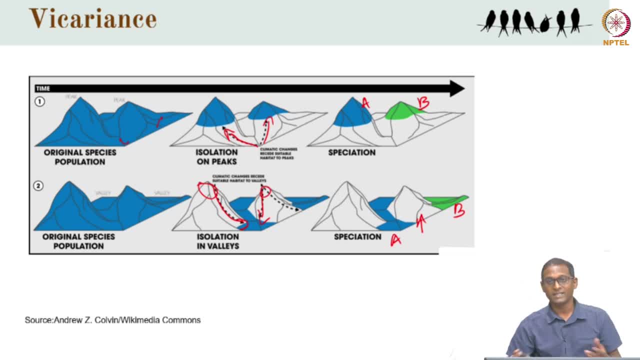 into a different area and then, I, gets isolated over a period of time, If you assume you know this species moving over to this mountain and then gets isolated. So that is, that is another mechanism of speciation in that is popularly kind of discussed in biogeography. 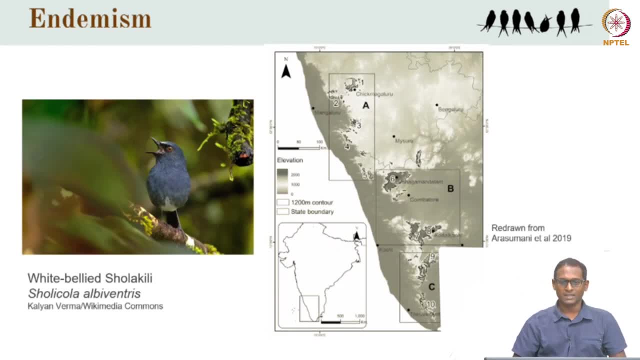 So all of this can result in high endemism, and one of the one of my favorite examples is of the white-bellied trollochillae, and this is found in the western Ghats. This is a map of the western Ghats and what you see against. 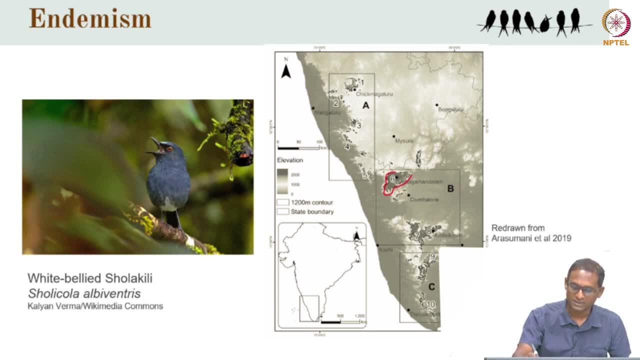 these numbers are mountains and this, for example- I am sorry my drawing is not very good, but that is the Nilgiris. you have the town of Ooty there and this here. you can see the similar contour here that has Kodai canal and Munnar, which is the Annamalais and Palni. 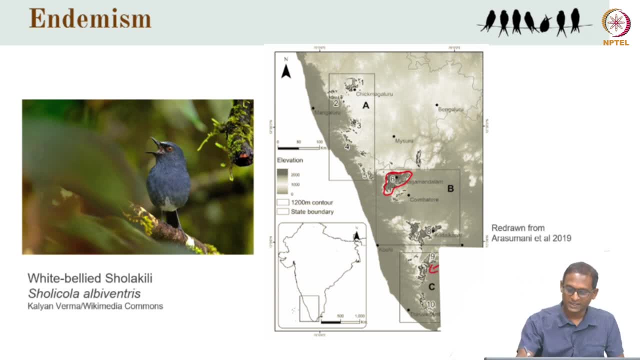 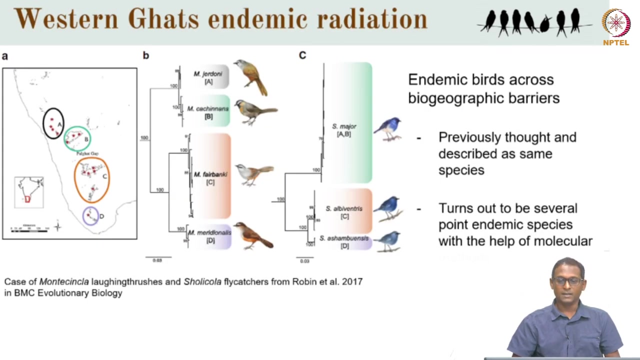 hills. then you have other mountains that are again isolated from each other. So these are all different isolated mountains, Yeah, and all of them have populations of this trollochillae right and earlier they were thought to be one species, but later we conducted a detailed genetic study and 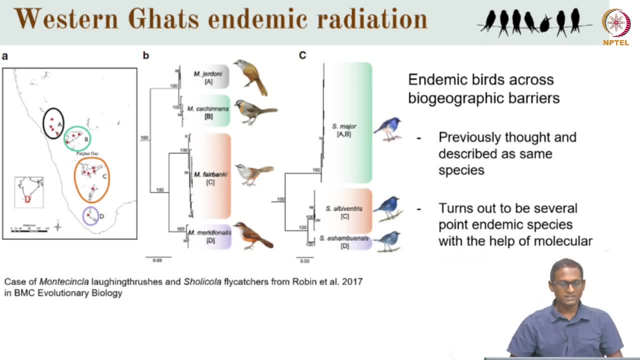 you know, we looked at plumage and we looked at song and we suggested that these are in fact different species. This was the case for the laughing thrush. So 1, 1, which is the Montes Sincla, these are the laughing thrushes and they are found. 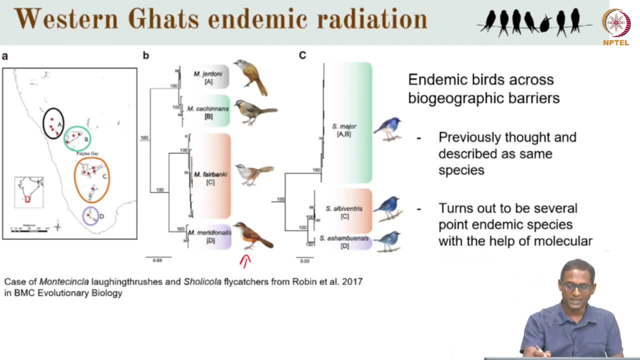 in 4 distinct locations, while the trollochillae are have 3 distinct species. So they formed- for sure, trollochillae A and B are that? you see here these 2 areas are very similar. So you see, essentially you see 3 groups, you see A and B, and then you see C, and then you see 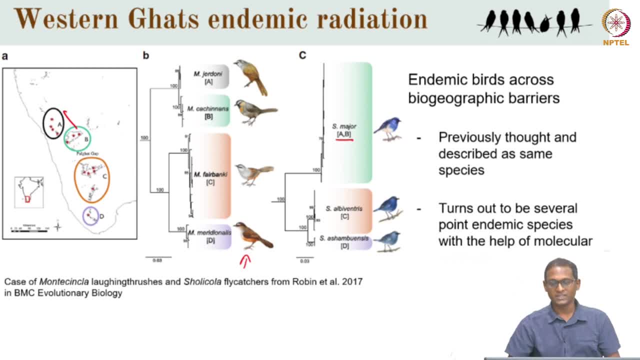 D And then type: if you simply click the capture here, you actually you see Saathuk and XZ, which-sooners, And we suggested that all three are different species and they are separated across the Palghat gap here by about 5 million years. yeah, and there is a similar divergence across. 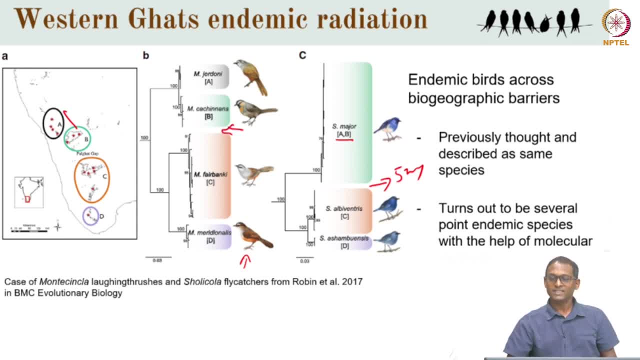 the Palghat gap for the laughing thrush as well. So these endemic species are separated across these mountains and these are now endemic mountain top restricted species found nowhere else in the world, and this obviously has implications for conservation as well. and this was found because we had molecular data- blood samples. 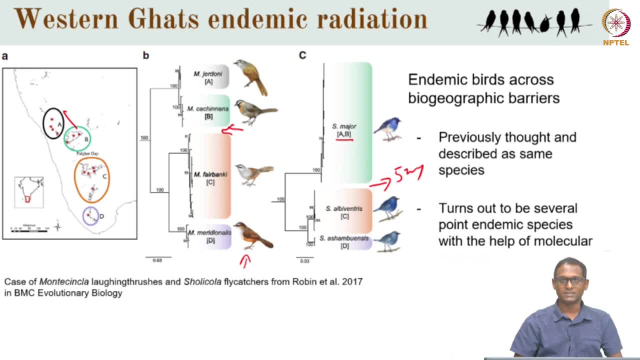 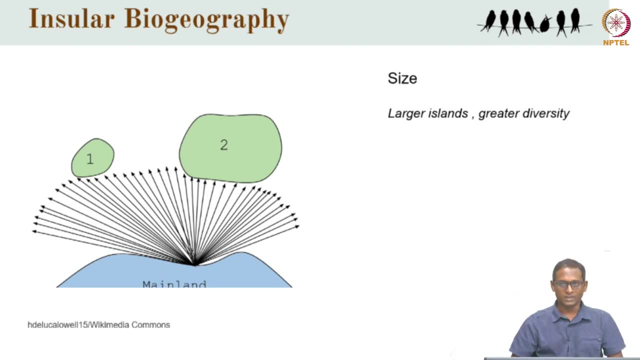 that we collected from birds in the wild from all of these different locations. Now we move to the idea of insular biogeography or island biogeography. This is a very important part of biogeography and sometimes it can be a little bit difficult. 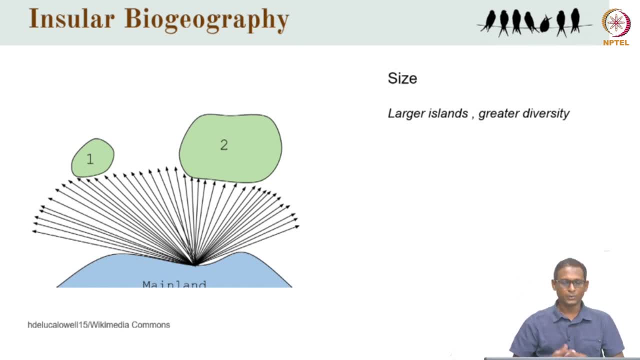 to understand. So I am going to illustrate this with a few cartoons and hopefully you can stay with me and you can understand the entire idea. So, essentially, the idea is that You have the mainland, which is here, and from the mainland species need to disperse, to get. 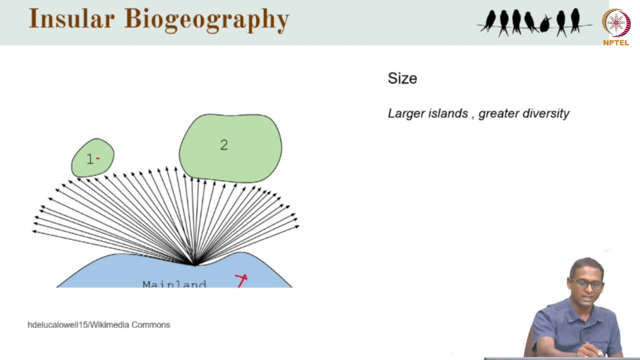 to different islands. and here there are two islands, island one and island two, and they are of different sizes: island one is small and island two is large. now, what happens is, as species kind of move out from here, they, you can imagine, you know, individuals kind of. 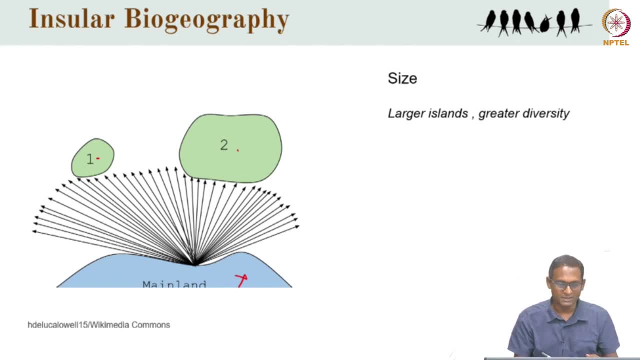 They are flying out from the mainland and the chances of them hitting a larger island is more, and essentially you see more colonization. given that they are at the same distance from the mainland, the larger island will tend to have greater diversity. there are other ideas that are, you know, that come into place for this. 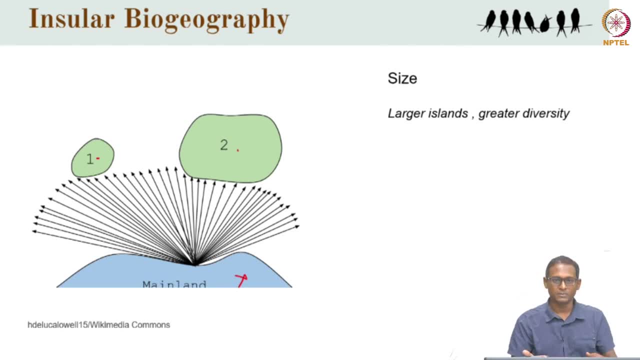 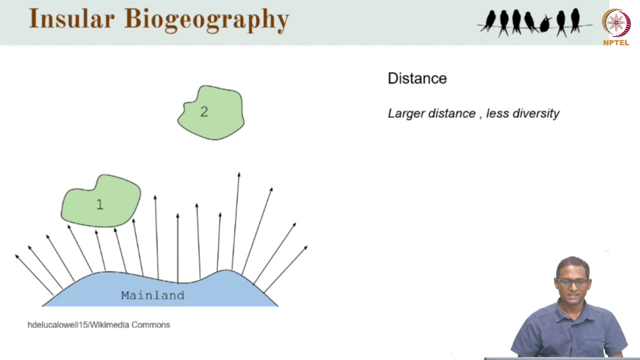 But this is an important idea as well. the distance from the mainland and the size of the island has an important consequence on the diversity of that island. Now you can also have similar sized island, like you see one and two here. they are the same size, but one is closer to the mainland than is two, and what you can see is that there. 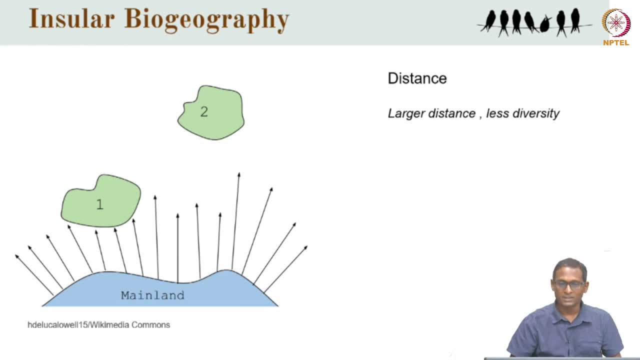 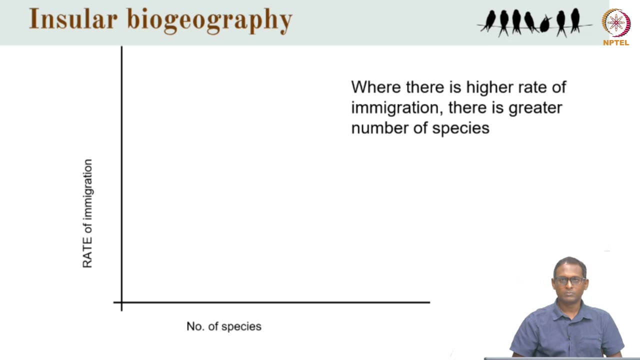 are probably more species that get to island one than two, So you Find fewer species in islands that are more distant from the mainland. so this is again a very important idea in biogeography. So to get to, there is an equation, there is a way that people look at distance and size. 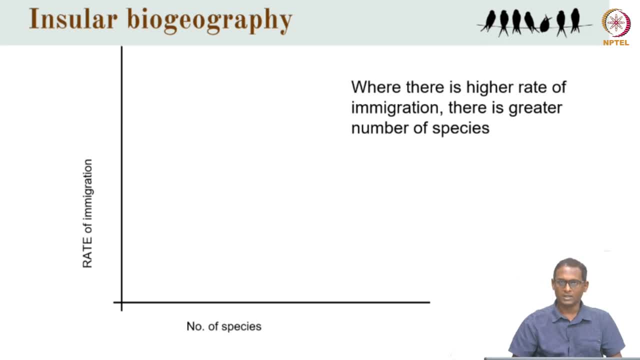 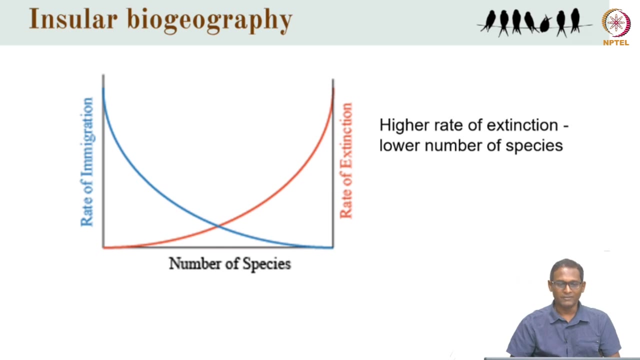 and how that affects the immigration and diversity. so if you have rate of immigration and number of species, The idea is that when there is more immigration there is greater number of species that come in. something like this, you can also have extinction here. so in this case, so in this case you have 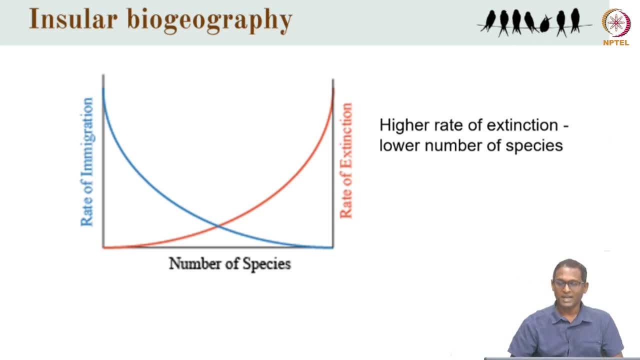 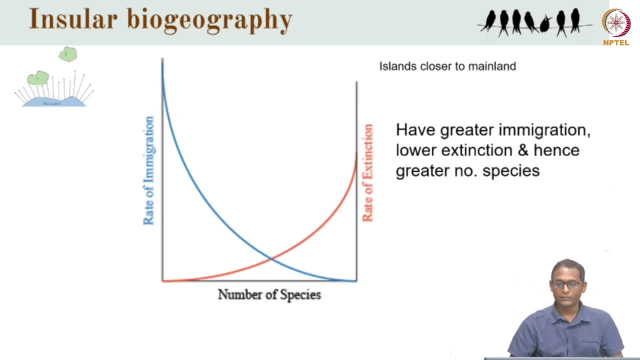 extinction on the other axis here, the rate of extinction, and higher the rate of extinction, the lower the number of species is. and if you remember that you, you know from our example earlier, the illustration that we had earlier, we know that for the islands that are closer to the mainland you will have greater immigration. so there is a skew in this line, that kind. 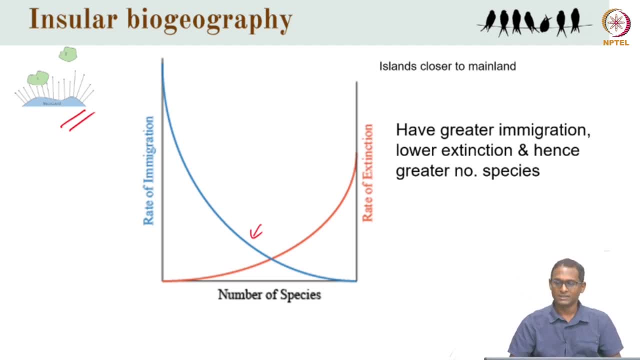 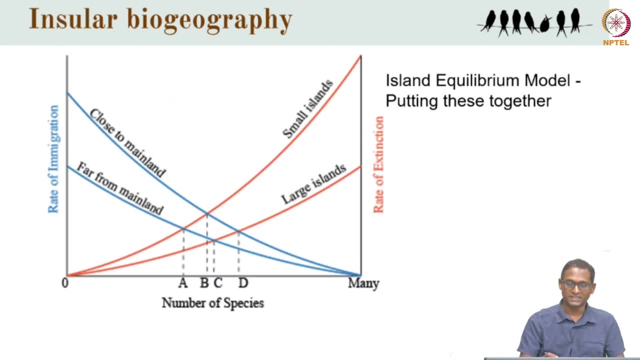 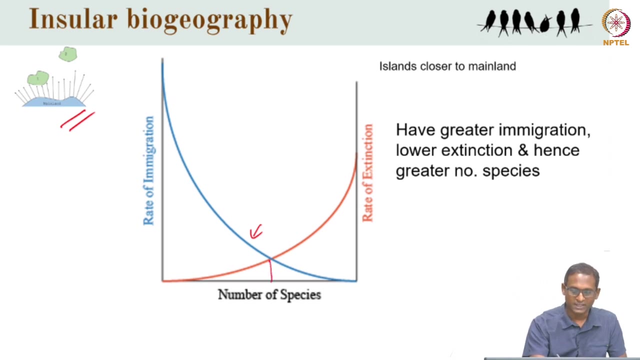 of pushes more immigration and lower extinction as a consequence also. So it will have greater number of species. so it will have a greater number of species and you get the number of species by kind of drawing a line here. so that is the number of species that you have at the intersection of the rate of immigration and the rate of. 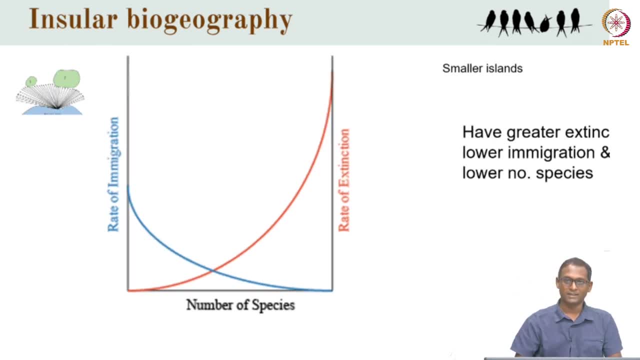 extinction. Now if you have a small island- again going back to the example that we looked at earlier, if you have small island, then your rate of immigration is lower, so you can see that here, but your rate of extinction is higher. number of species on the x axis is then a little bit less. yeah, So essentially you. 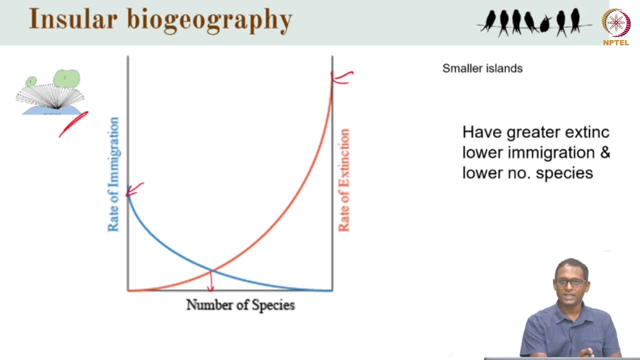 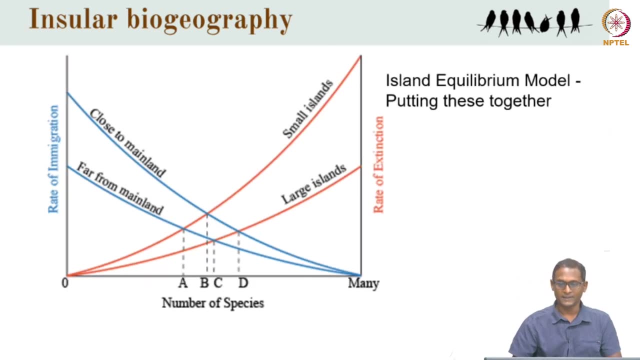 have to kind of imagine this interplay between immigration and extinction which has a consequence on the number of numbers of species at in that area. You can put these together and you get this island equilibrium model. So usually people get very confused with this, with the figure. but I hope that you can see that you have 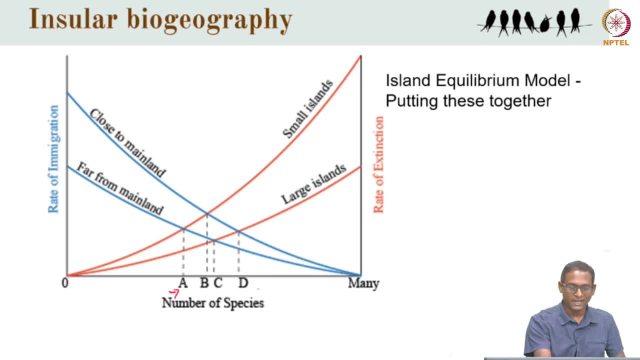 at least if you can get the A and the D, which is, if you are a small island and far from mainland- you remember that cartoon. If you are small and far, then you have lower number of species. and if you are a large island which is close to the mainland, which is here close to the mainland, then the number of species 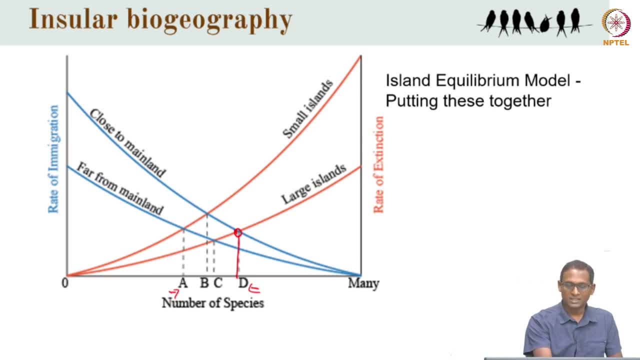 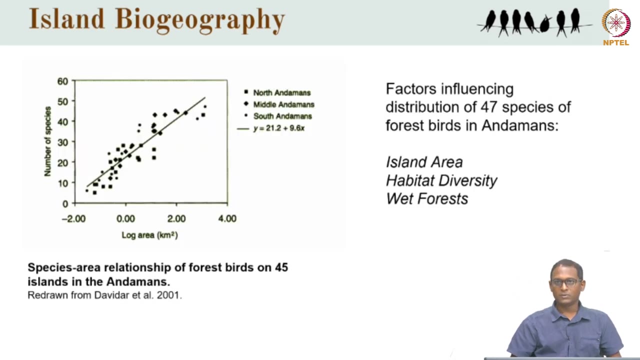 is more yeah, And of course, the between the B and C. things can change. it depends on a lot of other aspects as well, but essentially this is the. this is the island equilibrium model, to kind of put it simply. all right, So what do people find when they have a? 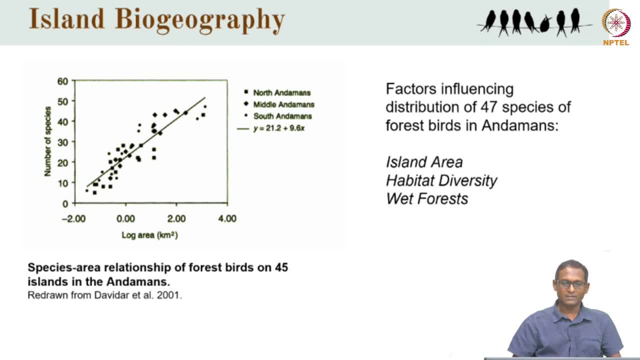 Have examined some of these relationships. Another important relationship in island biogeography is a species area relationship. This example is a wonderful example from Dr Priya Davidar's lab and they looked at birds in the Andaman islands and they looked at the distribution. 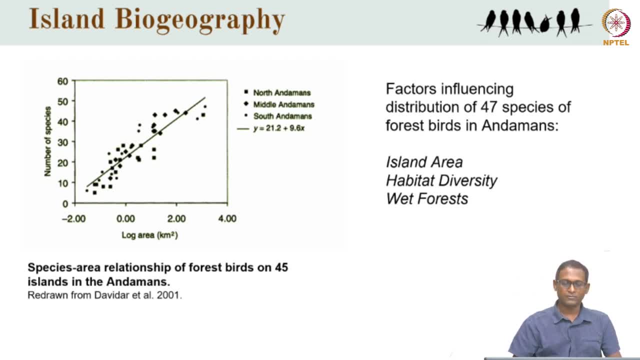 of 47 species of birds And essentially what they find is that there is there is an impact of area on the numbers of species, So greater the numbers of- sorry, the larger the area, the greater number of species that you find on an island, Of course. 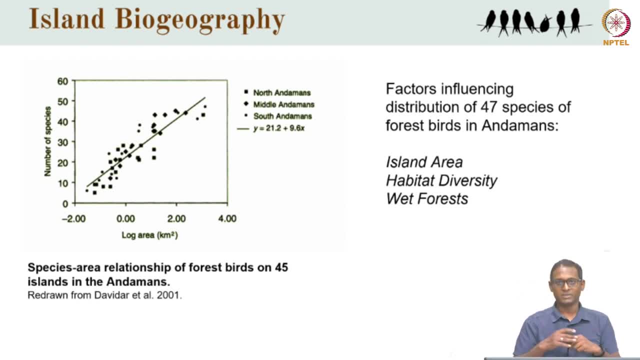 they also talk about not just the island area but the habitat diversity and the fact that you have wet forests that can support a large diversity. So there are other other aspects that that play. One of the fundamental things to remember is that larger the area, more niches, that that 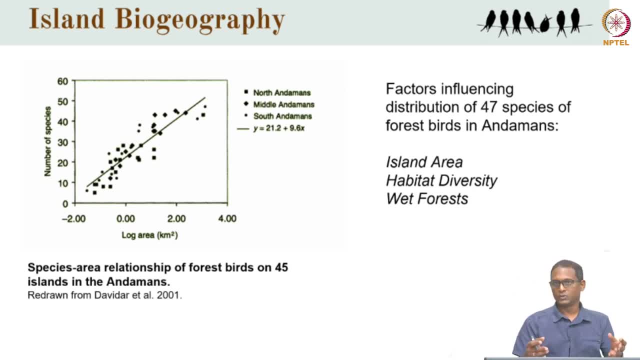 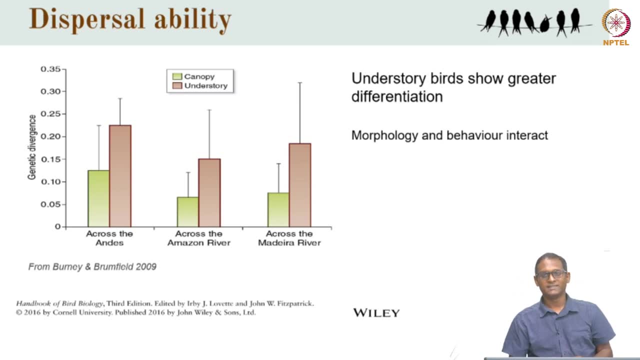 are there available for greater diversity. And then, of course, all the other island equilibrium ideas also come into play. In bio geography, one of the important things that people are beginning to understand is that the story is not the same for all kinds of species, especially birds, One of the concepts, one of the ideas that that people are talking. 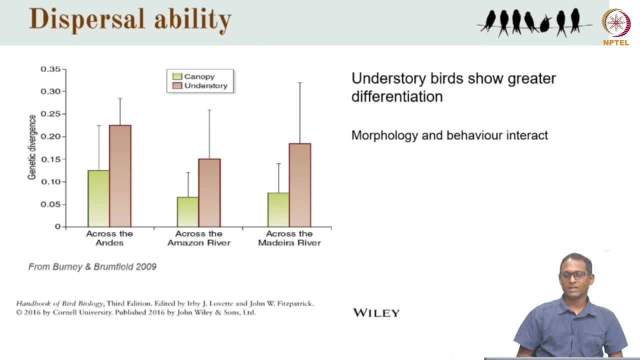 about More is about dispersal ability, which means how far can a species move, and we know that not all birds are alike. you have canopy birds. essentially, canopy birds are thought to, you know, look for resources which are more patchy and they can hence travel larger distances. this especially frugivorous canopy birds they track. 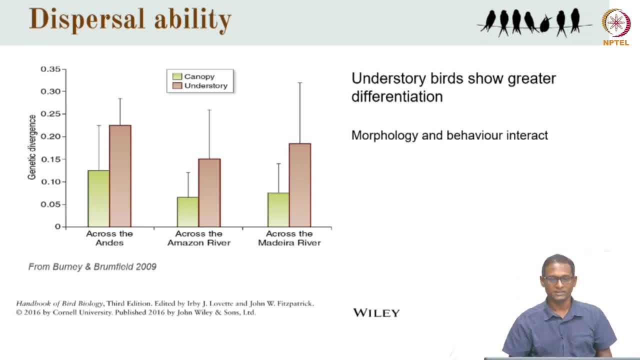 resources and they, you know, kind of move much farther and the hypothesis is that they hence they have lower genetic differentiation than understory insectivorous birds, which are generally sedentary. they are thought to be sedentary and this group of researchers actually examined that. 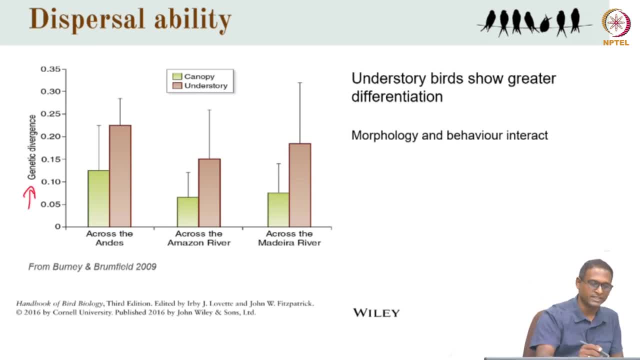 they looked at genetic divergence, which is which is here and across different barriers, like, for example, across the Andes, across the Amazon Or across another Madeira River, and what they found was across all of these barriers. they found that the understory birds actually showed more genetic divergence than canopy birds, which meant 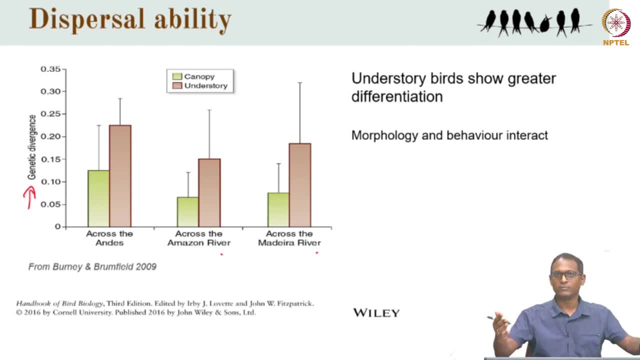 that the canopy birds were able to kind of move across these barriers much more than understory birds. so this is a very interesting aspect that a lot of researchers are beginning to kind of examine more deeply. And essentially it is not that it is just driven entirely by morphology. yes, morphology has a big role. 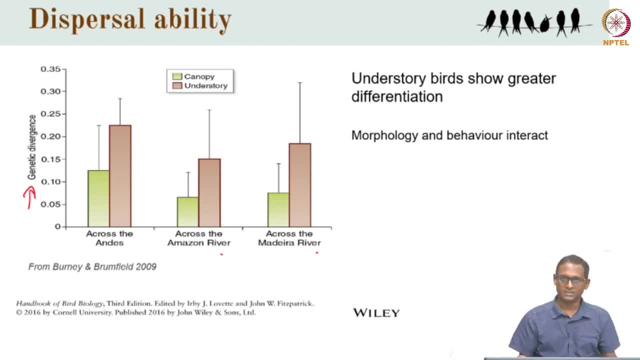 to play in it the shape of the birds wing or is one of an indicator. there is a hand wing index that people use as a surrogate of dispersal ability these days. so that is a good, a good, a good trait to use, but there is also a behavior. 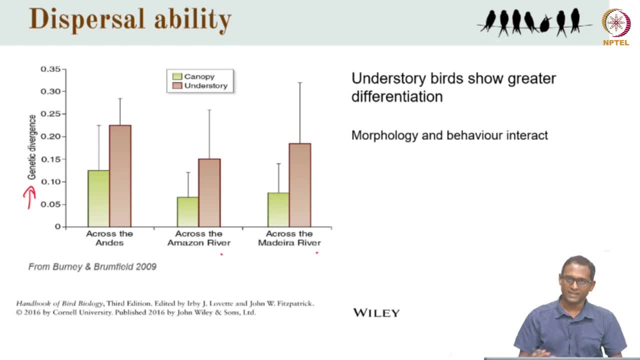 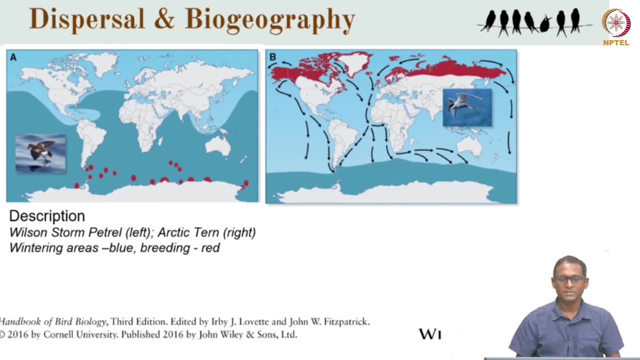 There is also a behavior. There is also a behavior And you know how birds actually interact with the landscape. are they tracking resources? the ecological aspect of it is also important in these biogeographic patterns that you see, and I just want to also give you an example of you know what happens to biogeography when these birds actually 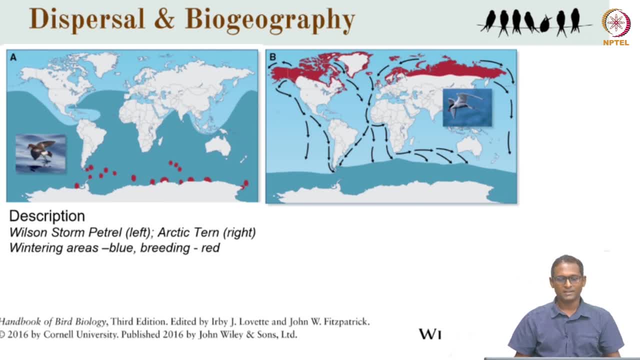 have very large dispersal areas and on the left here is the Wilson storm petrel and on the right is the Arctic turn And the areas in blue are the wintering areas and the areas in red which are kind of here and for these birds they are here. yeah, so those are. those are the breeding areas. but you can see that you know the these are. they are found all across the world and they move across the world. so obviously, when you are thinking of biogeography, you need to think about the 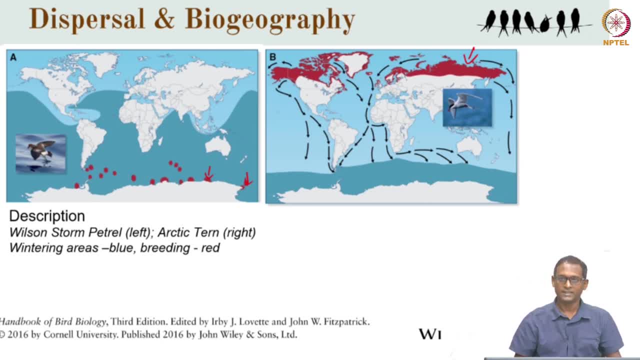 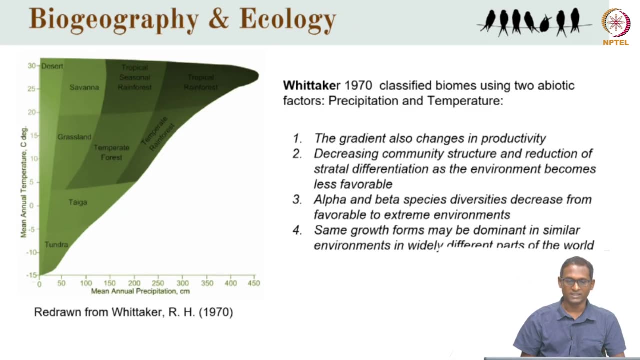 ecology of the species and how far they move. yeah, so these birds have very large dispersal distances And hence the biogeographic impacts would be would have to be considered accordingly. Another interplay of biogeography Is with ecology, and here 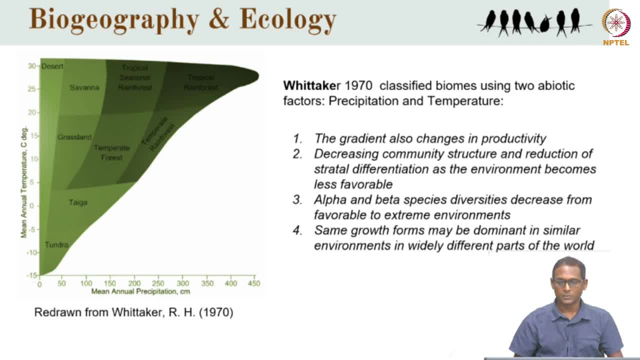 This is a famous diagram called you know. it was proposed by Whitaker in 1970 and he used two abiotic factors to classify biomes. Now, biomes are some forms of habitats and you have mean annual precipitation here, which is, you know, it goes from low to high and you have temperature going from low to high on. 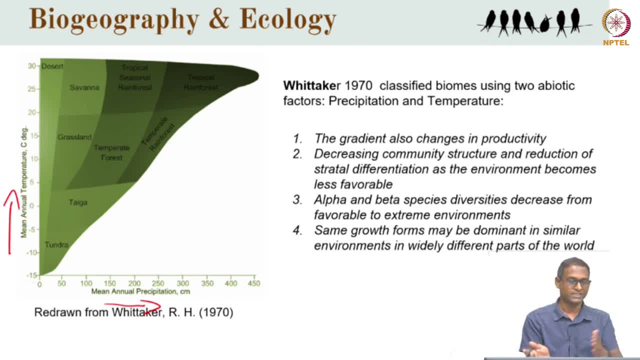 the y-axis. You can also switch this out and you can have precipitation on the other and temperature. you do find Whitaker diagrams that way as well. But essentially what the important part of this diagram is that you have some area which has high precipitation, which is here, and also high precipitation and high temperature. 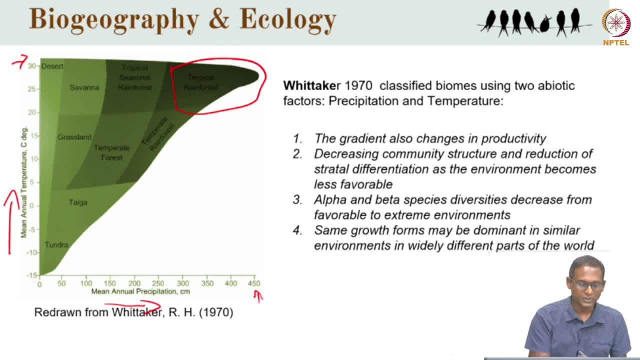 and those are the tropical rainforests. and then of course you have the tundra, which has low temperature And low precipitation, which is here, and in this case low precipitation and high temperature, which are the hot deserts right, And then a lot of the other habitats kind of fall in between this. 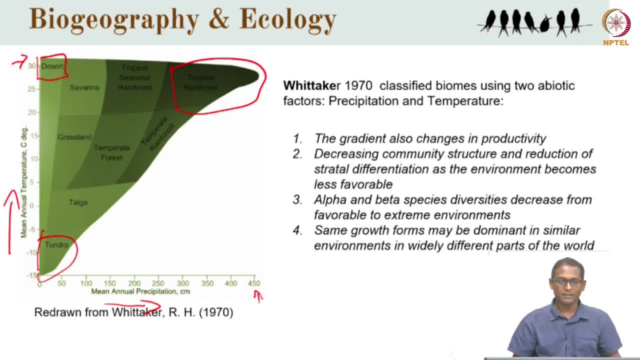 So this is a way to kind of explain diversity of habitats just using two abiotic factors: precipitation and temperature. So this is very elegant Now. it is also a gradient in productivity and you can find community structure changing, stratification changing and alpha and beta species diversity changes as you go from you. 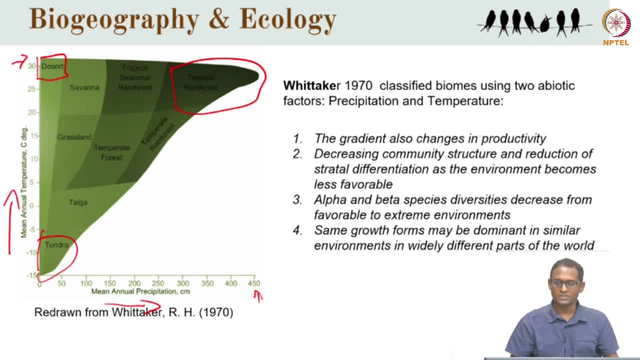 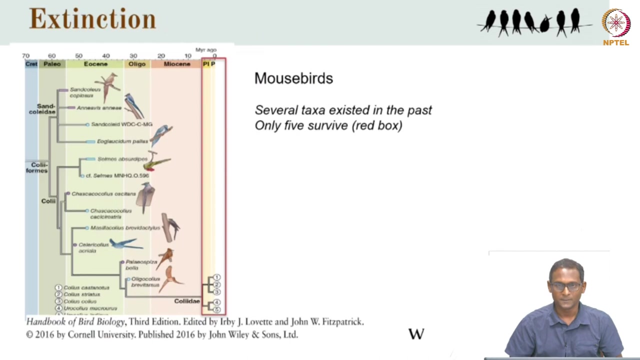 know, favorable to extreme environment and some growth forms are found in some parts of the world which have these habitats. So this is again another part of biodiversity Which looks at the interaction with ecology. This is a very famous and fundamental aspect as well. I want to. we did talk about- we talked previously about- the role of extinction, with respect. 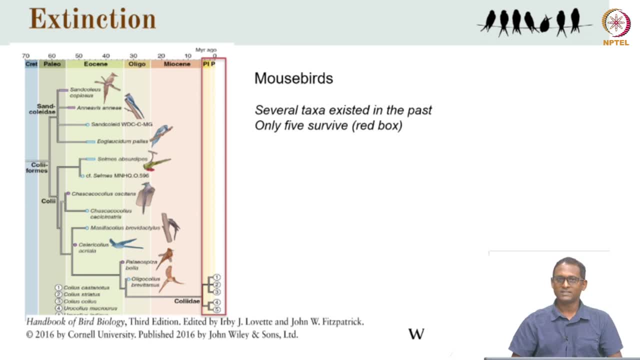 to relic species. I want to also stress a little bit more about the role of extinction in species diversity. Okay, And this is a very interesting example of this group called mouse birds, and we know today from various fossil data that several taxa existed in the past. and here again in 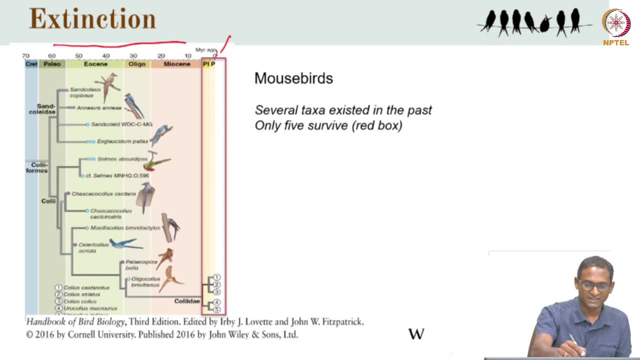 this graph, this is time and this is now, but so what is happening is, there are only these taxa that remain today, These five groups, Okay, Okay, Okay, These five groups of mouse birds. everything else is extinct, right So. so, essentially, what I am trying to say is that, when we look at species diversity, 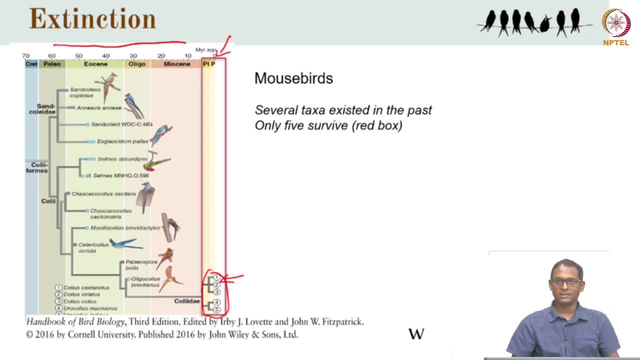 today. that may not be, you know, an indicator of how diversity has existed in the past. there is. there is a lot of extinction that has happened in the past and passerines. So there are very few studies that actually look at fossils and can look at how diversity 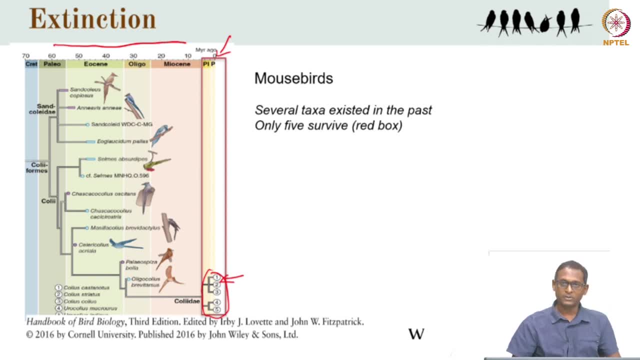 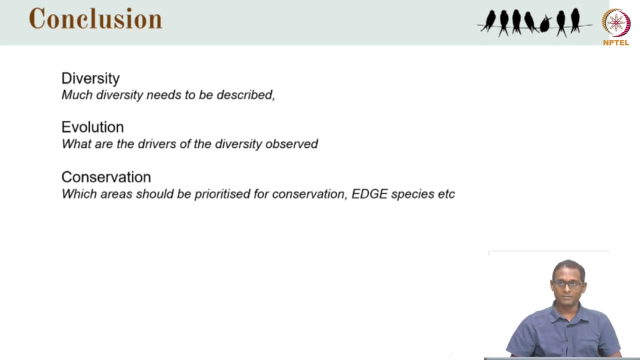 was in the past. So what we are seeing today is only a snapshot of diversity that has managed to survive through fairly long period of time. So, in conclusion, Okay, Okay, Okay. So biography is about understanding diversity, and there is much diversity that needs to. 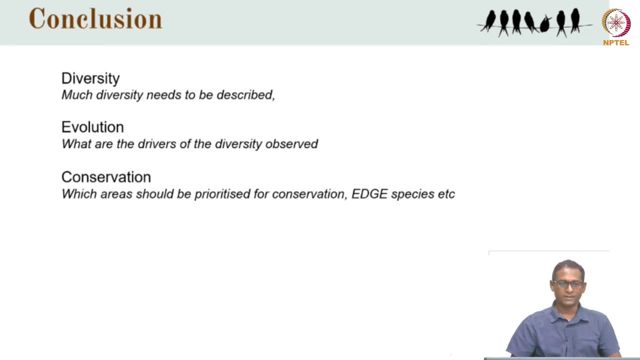 be described, especially in a country like India, where phylogenetic studies- phylogenetic studies- are very limited. There are very few studies on evolution to understand what are the drivers of these biodiversity, how our, where do species originate from? how do they colonize and move? these are again. 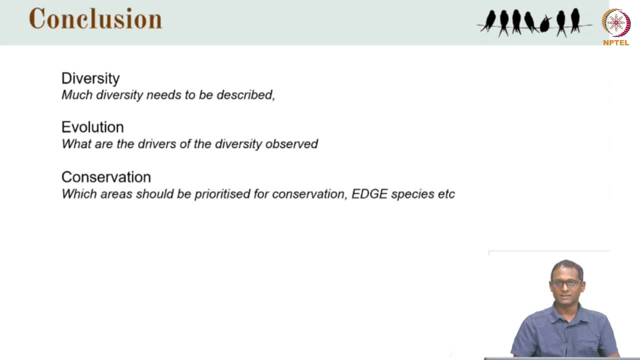 very fundamental, Fundamental questions that remain to be answered in the Indian scenario: conservation, of course, biography has a big role in conservation as well- and some biographic ideas, biographic realms, how biodiversity is divided across space and how they are connected- that can be used for conservation prioritization.